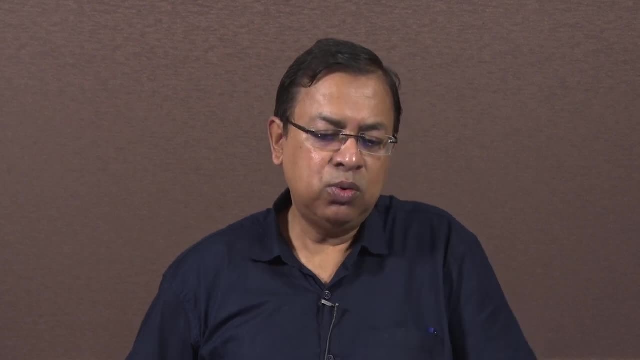 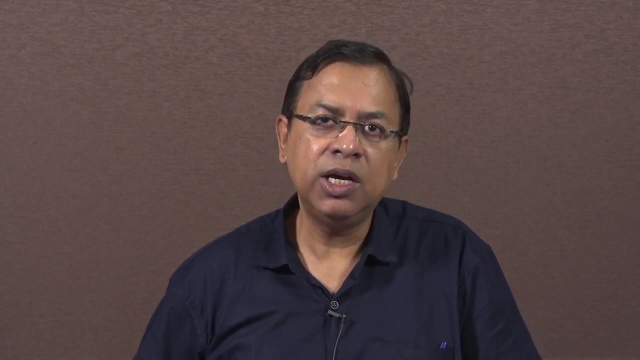 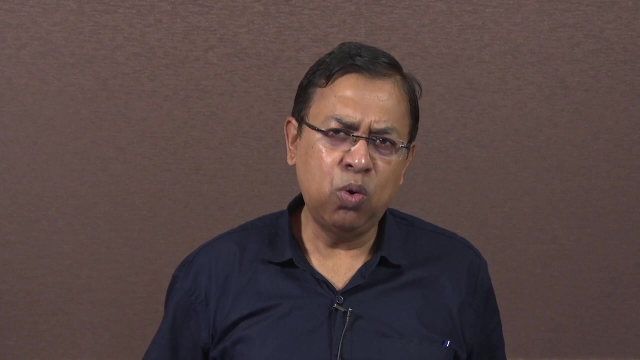 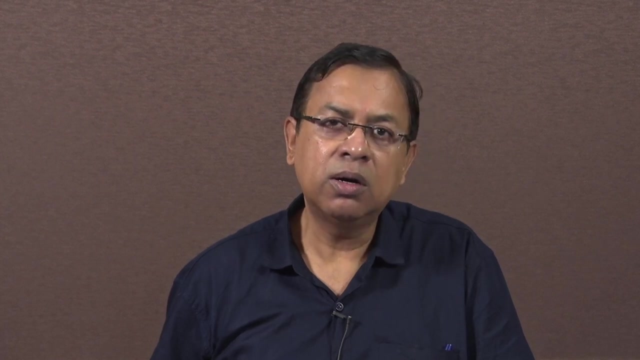 We will not get into what he exactly wanted to mean by this, but there are far reaching consequences of this topology in various branches of physics, which is what we shall elaborate here. So it is known for a reasonably long time that topology may have significant bearing on classifying systems, and the way it occurs is that we know that there are systems. 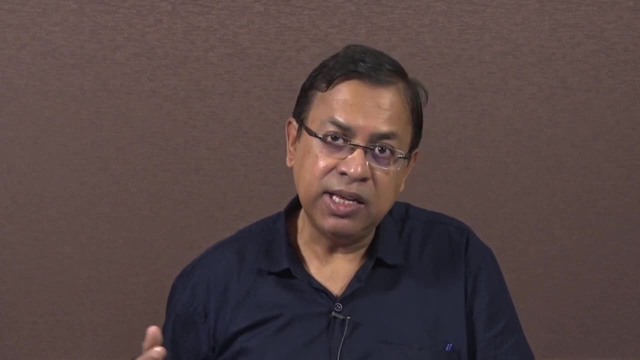 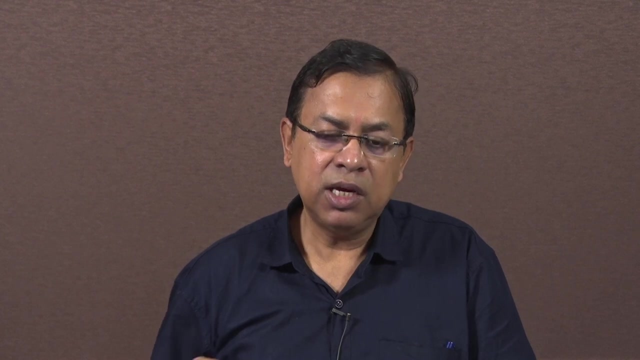 which have these singularities that appear in the system And these singularities in certain systems they appear as vertices or vortex, and these vortex is something that it is like complex numbers: Z equal to r, exponential i, theta. so when theta goes from 0 to 2 Pi, these complex number remains unchanged. So there is sort. 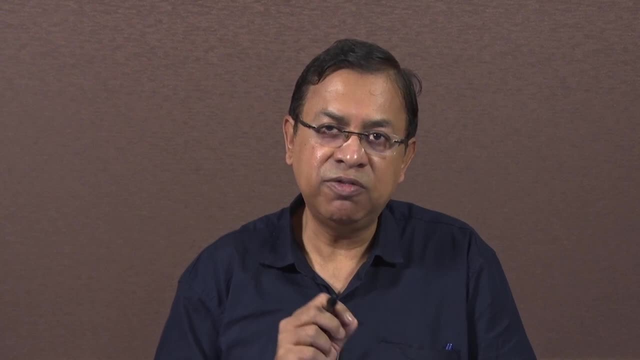 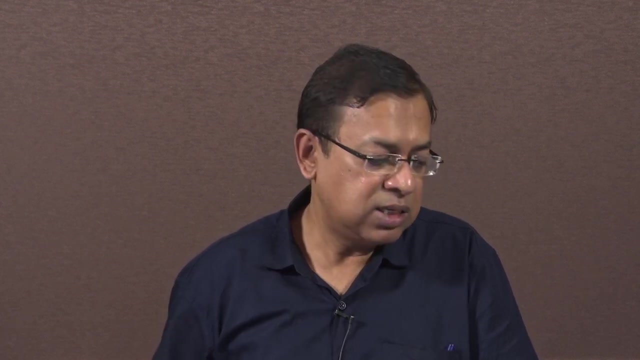 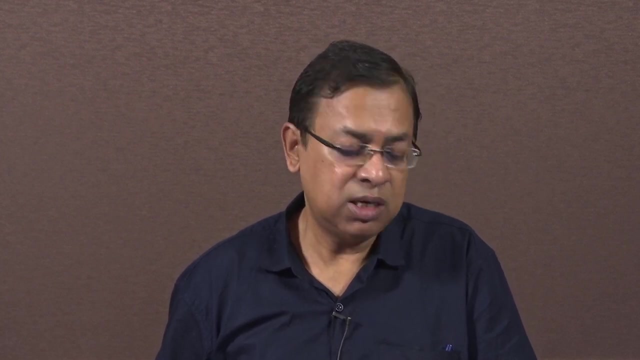 of the centre or the origin of this definition of complex number is where a vortex resides. So the focus is that, whether you know, these vortices can be contracted to a point without crossing each other, that is, without crossing one vortex, and this branch of mathematics, which now has entered significantly, 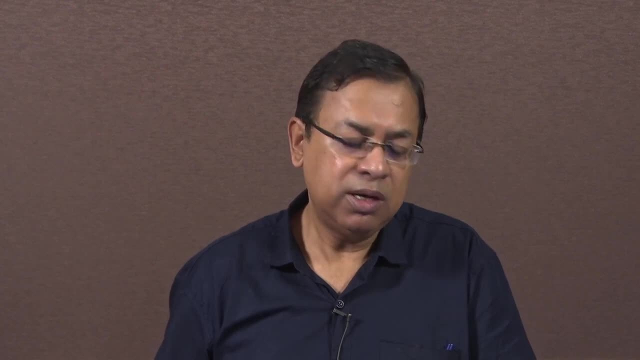 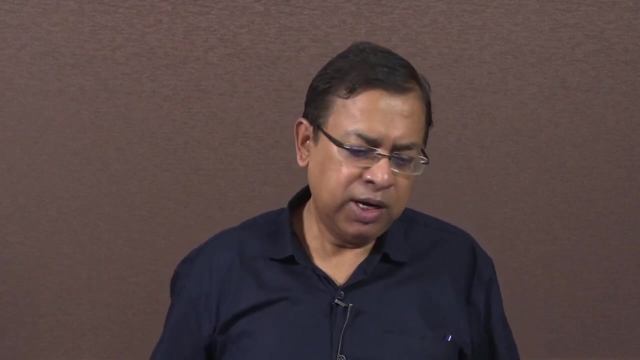 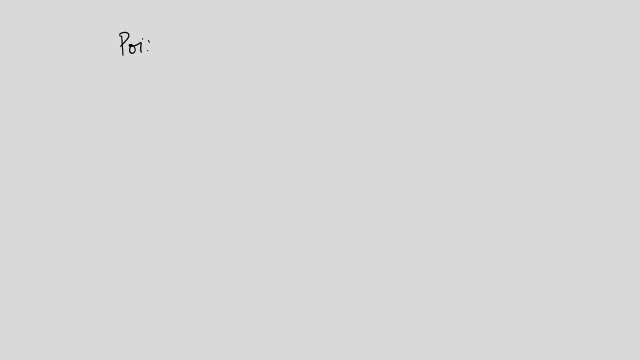 into physics, which is called as a homotopy theory, and it plays a very important role in algebraic topology. all right, So Poincare started all these studies, and so all these things started roughly about the end of the 19th century, which is 1898. 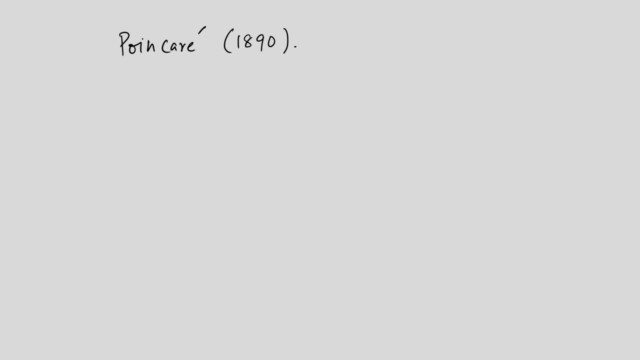 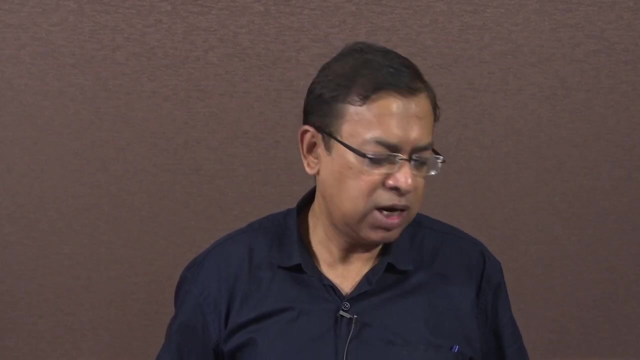 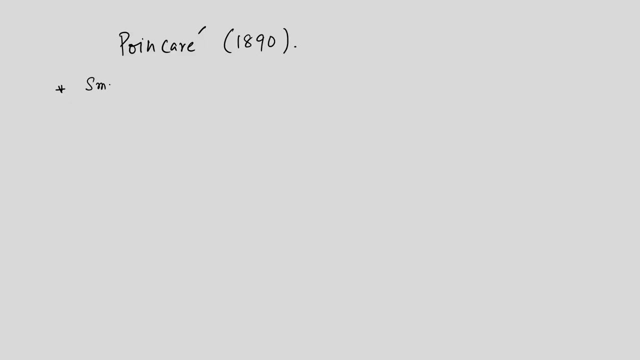 and so on, and so, while investigating problems in celestial mechanics, which is popularly known as classical mechanics in the modern times. So there are a few things that he noted. one is the smooth mapping between the surfaces. second is there are these fixed point theorems, and then there are the singularities of the vector. 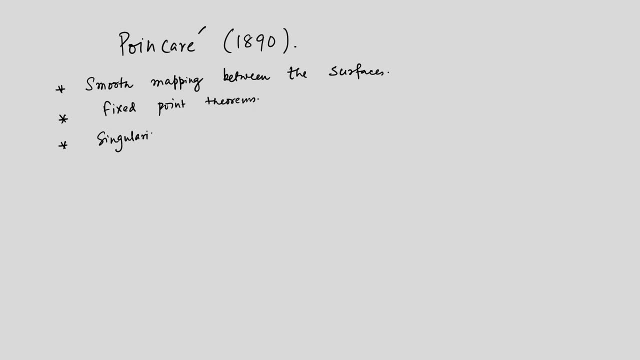 fields. So he pointed out that the structure of this topology is really that these вот click patterns in the topology features, the 그런데 of the strata of the topology of the six point philanthropic systems and two of the three other types of topology. of the three other types of topology, the two: of the three other types of topology, of the four times geht- or the four times get-, and which you can also find in the Karmann and the syntactic systems. There may be a lot more. So these are really the applications of topology in physics. 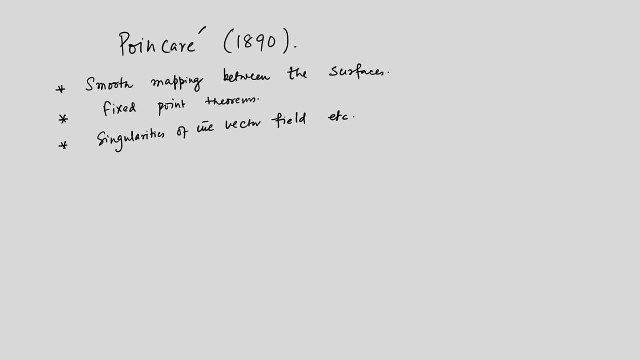 Poincare. so he sort of pointed out that these results of these, they can be systematically applied to other mechanical systems, electromagnetic systems, optical systems, in particular acoustic systems, and so on. Now is this very new, is this something that we have never been aware of? these applications, 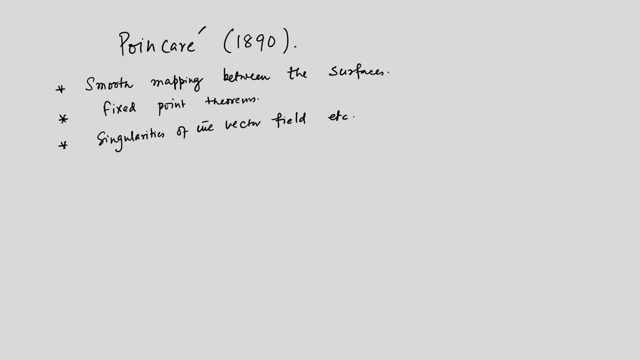 of topology. in physics say for example- and it is not that I mean, if you really think about this, Gauss's law, let me write that- and Ampere's law in standard electromagnetics. So this was E. dot ds is equal to Q enclosed by epsilon 0, and it is a closed surface integral. 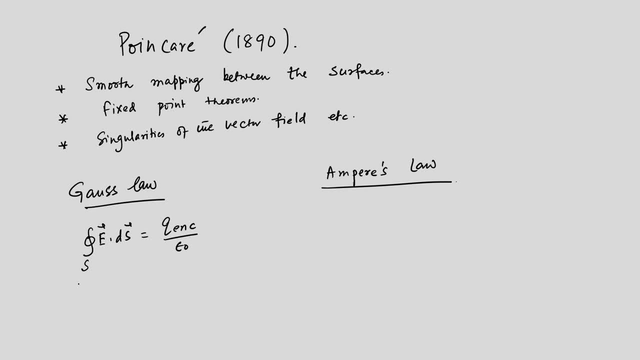 and this is the surface. This is a. we sort of call it as S, and also B dot dl with where B is the magnetic field, here is the electric field, So flux of the electric field, and this is like the line integral of the magnetic field, is like mu 0. I enclosed sort of for convenience. I am taking it to. 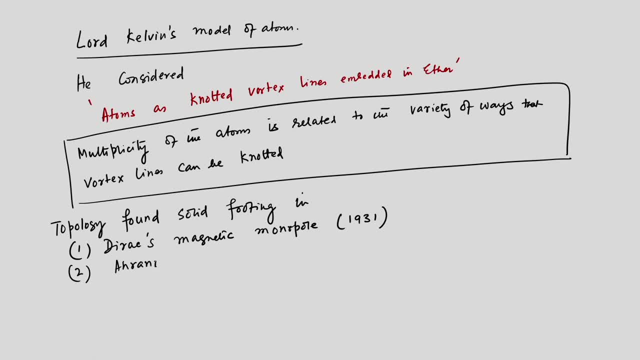 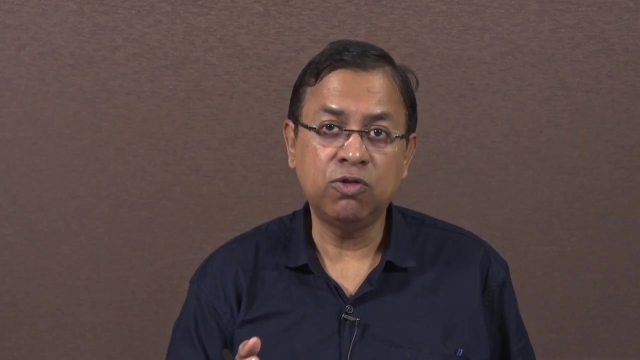 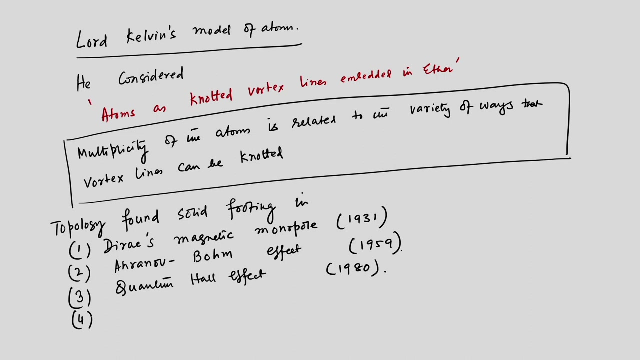 Bohm effect, That is, oder, if there is an upbound effect, which are just phenomena. quantum Hall effect is the first realization that Budie electron gas, in presence of a strong magnetic field, can be considered as a topological insulator, and this was the first realization of quantum. 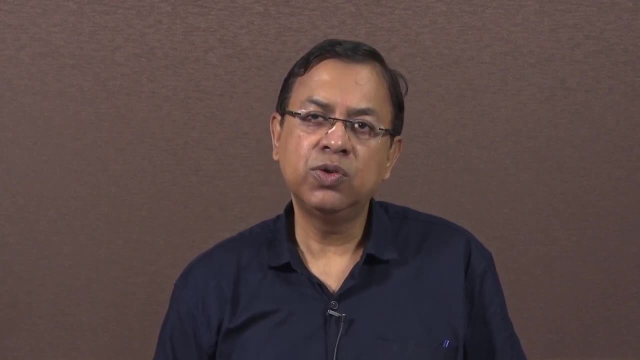 or a rather topological insulator, which was in 1980.. topological insulator with spin filtered edge modes, etcetera. they were discovered in 2005 and they were they found to have a lot of applications in very interesting phenomena called as a spintronics, which in principle could replace the electronics and would be 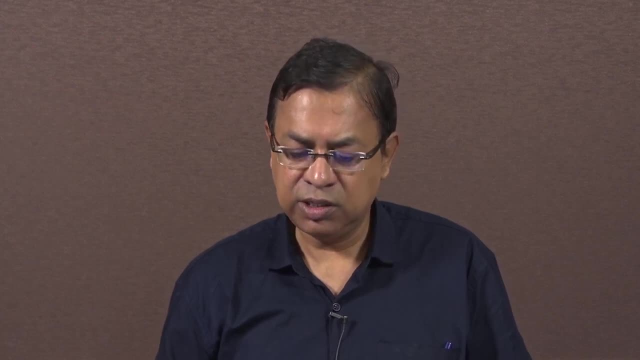 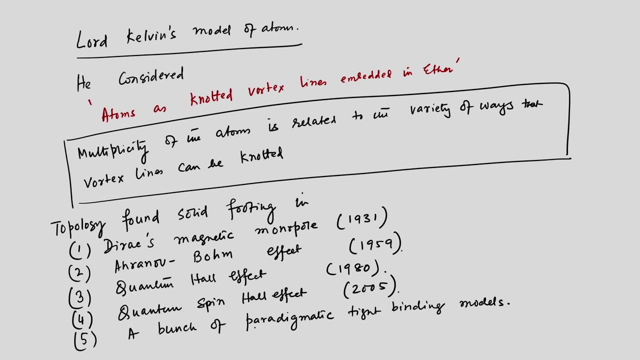 a next generation devices, communication devices and so on, and we will talk about, you know, three, four and as well five, where we would talk about a number of models which are very simple models, yet they capture the topological properties in a very systematic way and we can, because of these are tight, binding models, so they can be written down nicely in case. 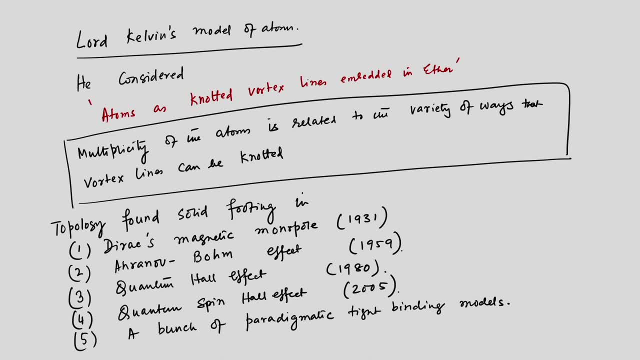 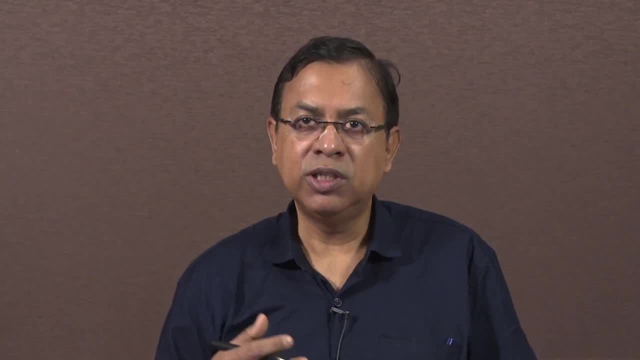 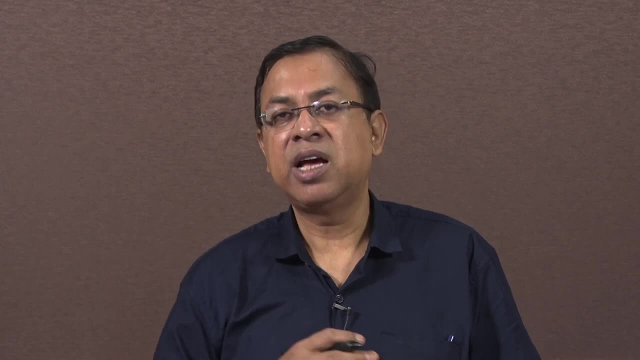 space. So we can calculate the topological invariant and we can show that when the system sort of makes a transition from a topological phase to a trivial phase or vice versa, or from one topological phase to a different topological phase that are characterized by different 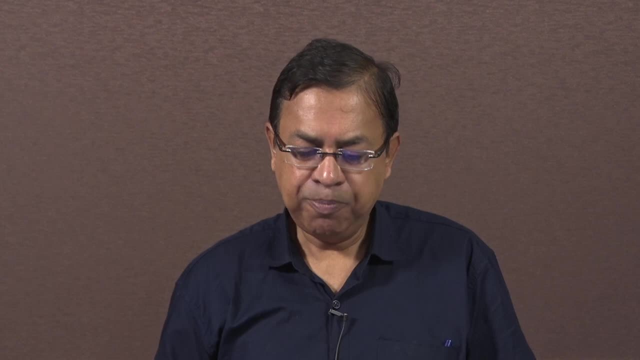 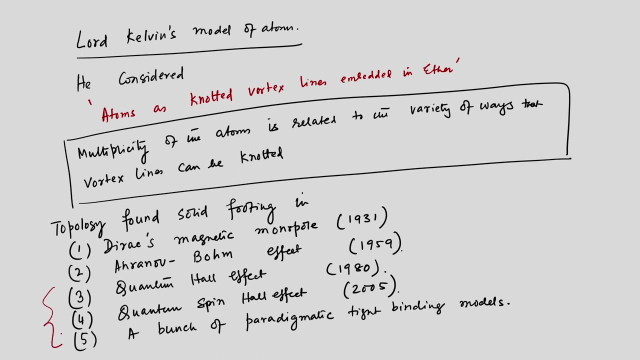 values of the topological invariant. So we will talk about these three in details throughout the course. However, just to make matters complete, let me discuss these Dirac's magnetic monopole and Aronoff-Bohm effect in very brief, so that one gets an idea that which are, as you see, 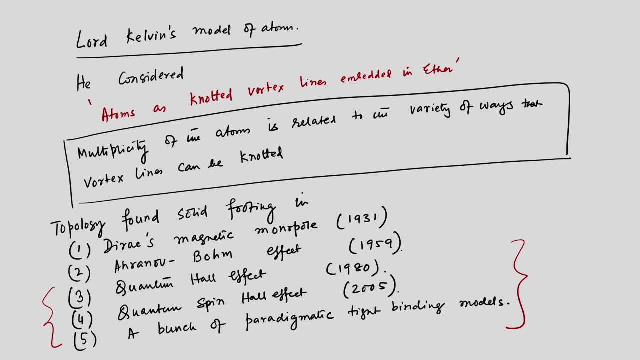 that, chronologically, they occurred much before the quantum Hall effect. and these arguments are very elegant and they are definitely worth seeing in this context. However, we will not sort of deliberate on them too much and we will go on to this. actual studies of topology in condensed matter physics, whereas these, the first two, actually correspond. 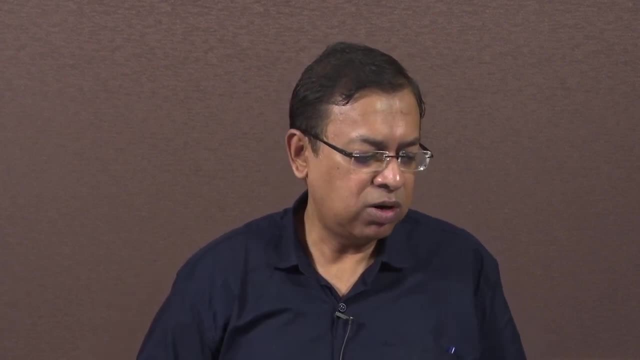 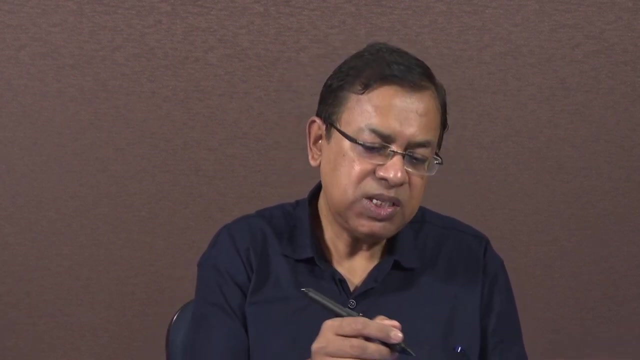 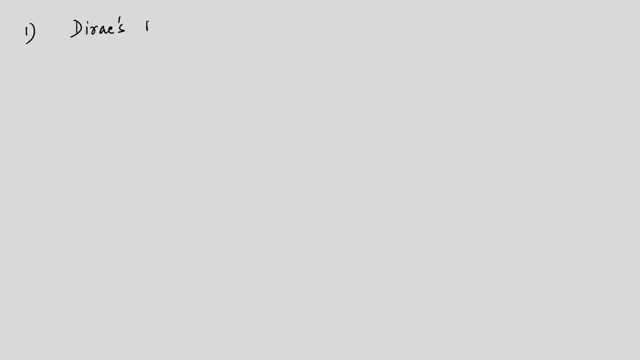 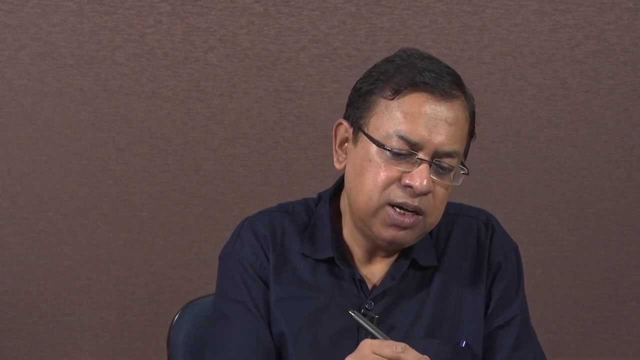 to any general physics in particular, say quantum physics or electrodynamics say, for example. So let us talk about these Dirac monopoles. So suppose there is a monopole that exists. so it is like a point like magnetic charge, and if that would create a magnetic field. 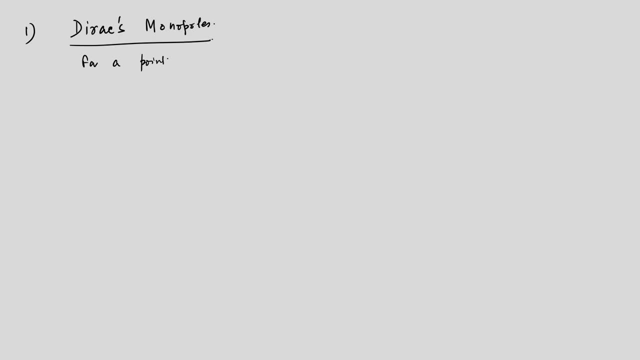 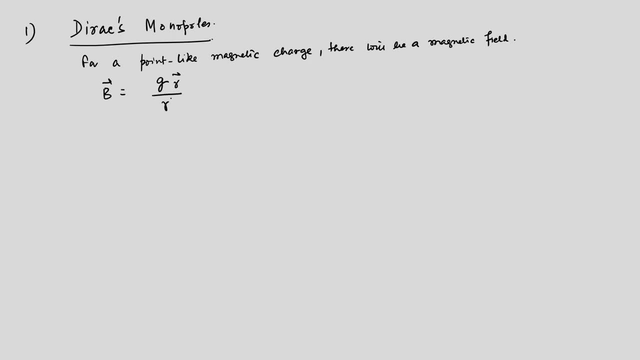 magnetic charge and let us write down this as R by R cube, which would be represented it by a potential which is given by this, and this is as opposed to a vector potential. this is a scalar potential which depends upon the vector r and if we want to reduce the complexities, 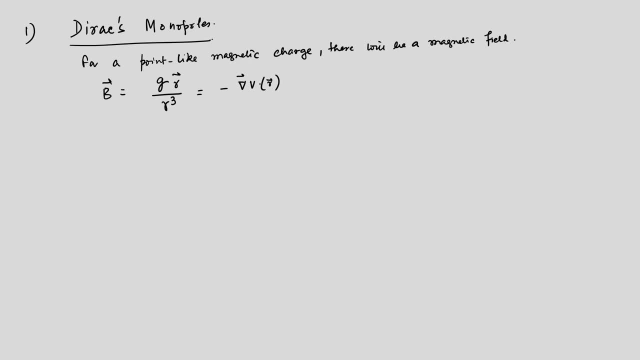 then these r can simply be the vector, r can simply be just r and not a vector, which means that it has no dependence on the angular variables theta and phi. okay, So g is the magnetic charge and V would be simply equal to. so V of r will be equal to. 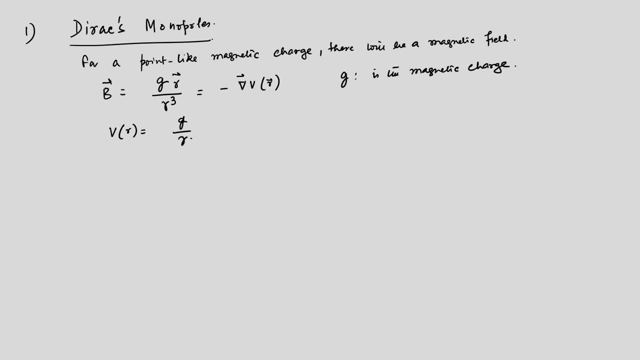 g over r and then. so this is, you know, because of this identity, that the Laplacian of 1 over r, Laplacian of that, and this is equal to minus 4 pi, delta cube r, and this is Dirac delta function in 3 dimension, and this is the Laplacian of 1 over r. This must be a known result in 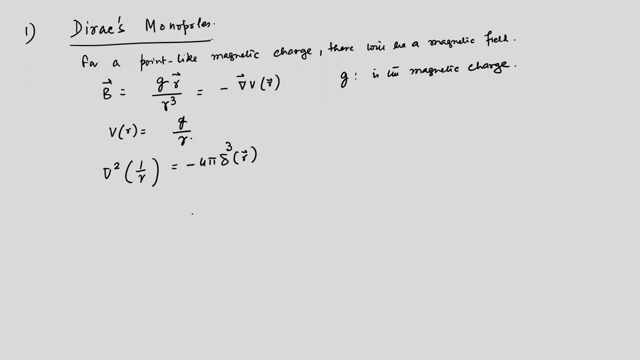 electrodynamics. So what it tells you is that these, if you take these things, if you take the Laplacian, that is del square, and operate it on 1 over r, it will give you zero contribution everywhere, excepting at r equal to 0. So that is why this delta function. 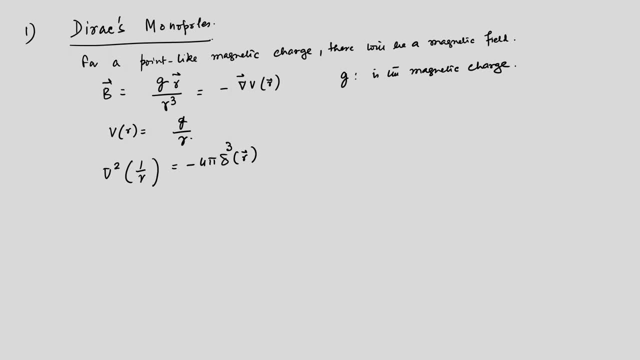 comes, and because we are talking about 3 dimensions, say spherical polar coordinates, so it is a delta cube r. So then the magnetic analogue of Gauss's law becomes equal to divergence of B, is equal to a, 4. 4 pi g delta cube r. So that is like the Gauss's law that we are aware of. Now you 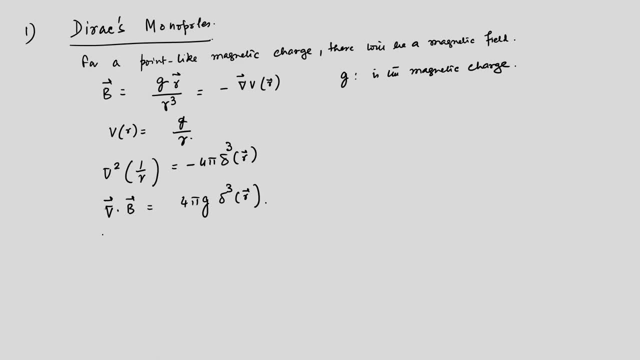 know what happens when you have a magnetic field to be present, the wave function of the particle that evolves, So usual, you know the wave function sort of can be represented as if p is a good quantum number, You know k is a good quantum number, It is represented by this. But in presence of a 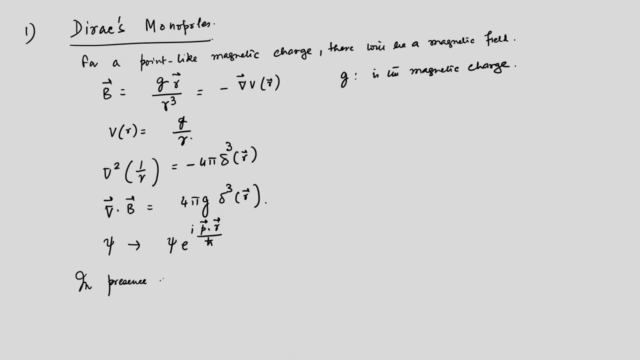 magnetic field, p is actually p minus e, a, where a is the vector potential corresponding to the field. Now, in Literature you might see a c. I will leave you with the dá. You might think that, okay, you could see a c. is this vector? No, that is just randomζ is equal to the C. Therefore, 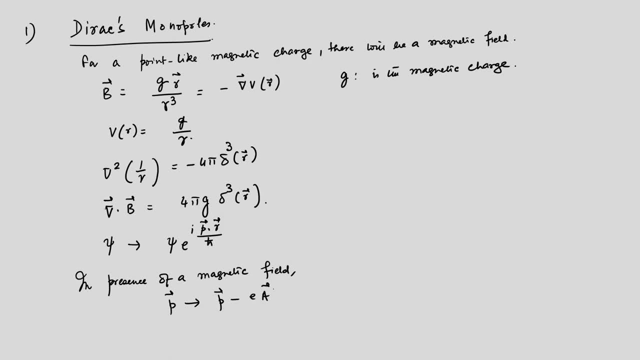 below, which is actually in Gaussian unit, we want to write down in the SI unit. So now, because of this, there is a phase difference. if a particle you know sort of goes from, let me write it here itself. If particle goes from point A to point B, it picks up a phase. 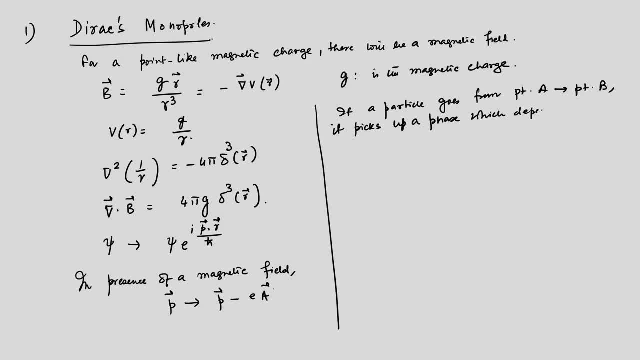 which is upon the path. So remember, if there is no magnetic field, then these phase that you see is not a path dependent phase. However, this picks up a path dependence phase and which this called as a minimal coupling, or the Piles coupling, and this phase is given. 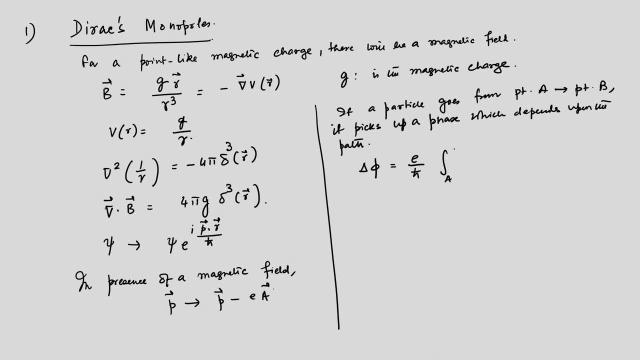 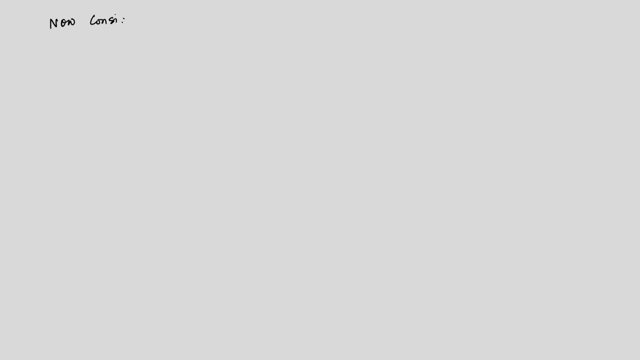 by E, by h cross and A to B. So here we have a point B A R dot D L, where D L is a vector that connects the point A to B. So D L connects A to B. these points Now consider a closed loop. So this is a closed. 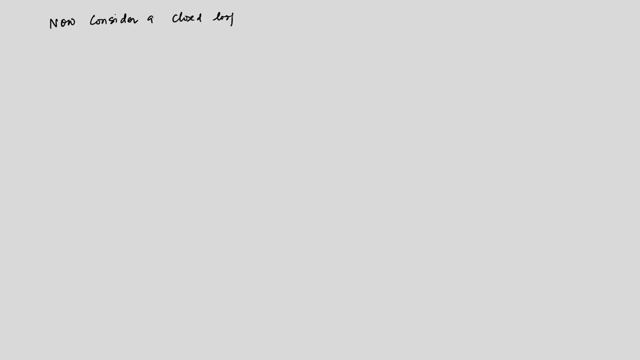 loop. So we will write down Gauss law, So the Gauss law which we have written down just a while back, So this Gauss law will give us a potential. This is: this is basically the flux of the electric field. So E dot. 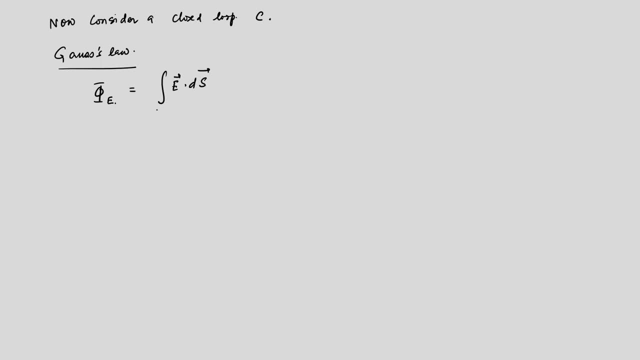 ds, E dot ds, and this is over S and this is nothing, but let us just call it as, because we are talking about electrons and or the electric charge and this. so let us write E over epsilon 0 and similarly for the Ampere's law, which will write it as phi B, this is: 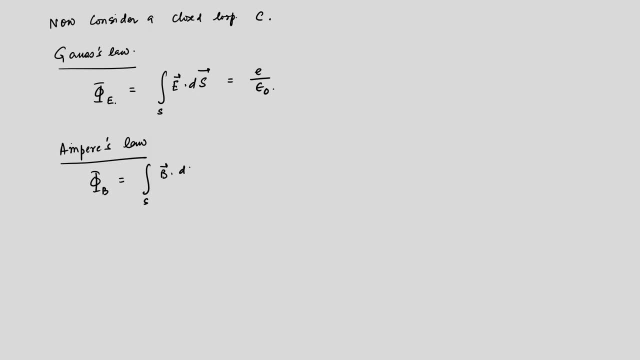 equal to S and B dot D say, for example, S again. So that is this, which is nothing. but if there is a monopole then this will be like G b over mu 0. So S is any surface which is bounded by this C. 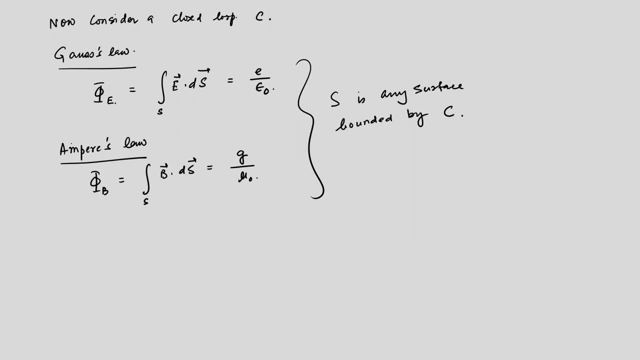 So as the particle it is transported around this loop, which is this closed loop C, then it will sort of this magnetic flux say, for example. so particularly we are talking about this flux for a closed loop is nothing, but it is like E over h cross, then it is Ar dot. 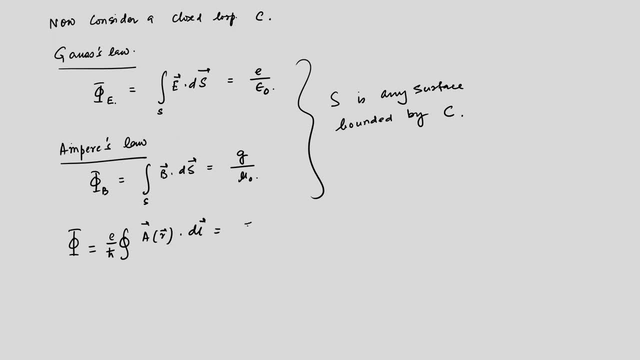 dl And this is equal To E over h cross. we apply Stokes theorem and Stokes theorem says that A dot dl or the line integral of any vector is equal to the curl of that vector and the corresponding surface integral, where the surface actually is just like this, that it is bounded by this. 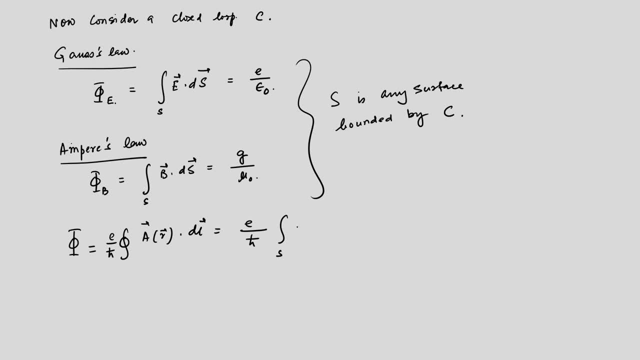 closed curve C. So this is equal to B dot ds and this is nothing but E by h cross, And this is a phi, which is a b. So this is that b dot ds, which is what we have defined as flux of the magnetic field. So we are just assuming that there is a magnetic monopole. 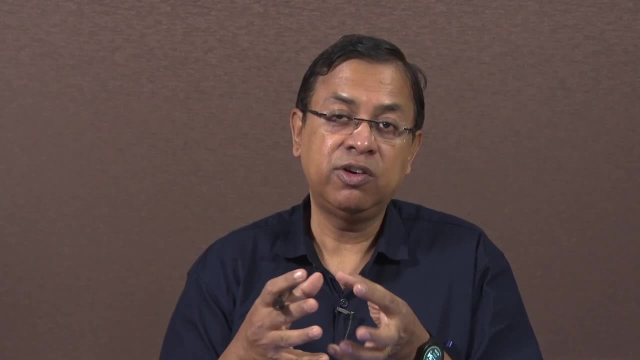 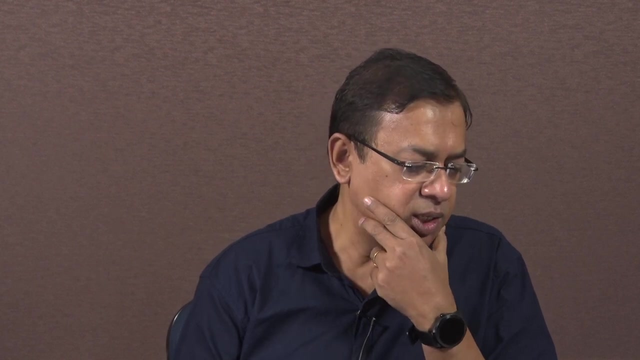 that exists, and the description of the electric field and the magnetic field are in the same footing, and that is why we can write down this. So now talk about the wave function of the particle. So let us see what is the wave function of the particle. So let us 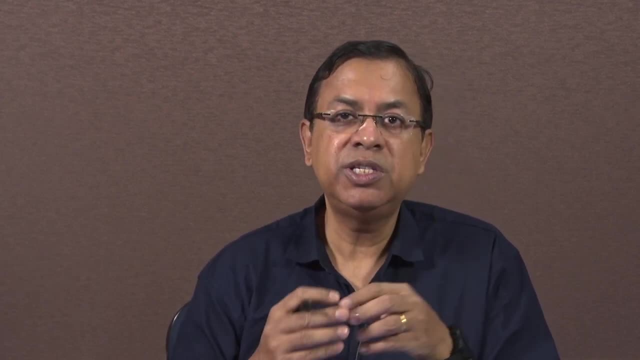 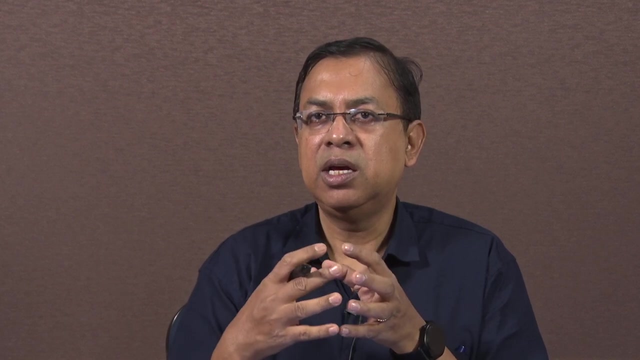 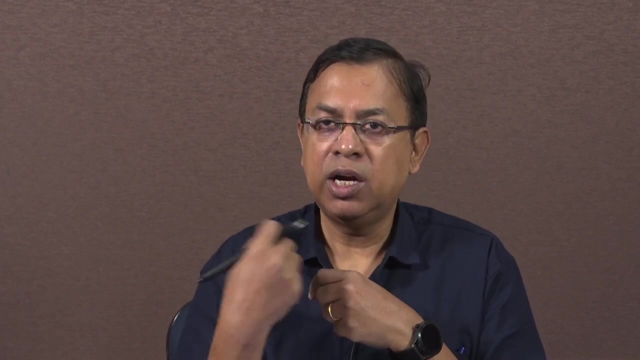 of the particle. So the wave function needs to be single valued, which means that if you take the wave function over a closed loop, then there is no effective phase that it picks up- we are not talking about the dynamical phase- but over that complete circle it will. 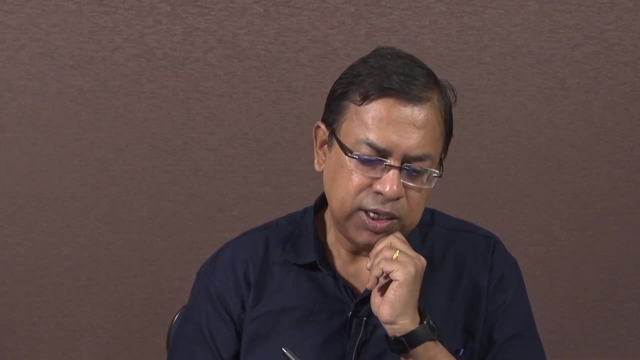 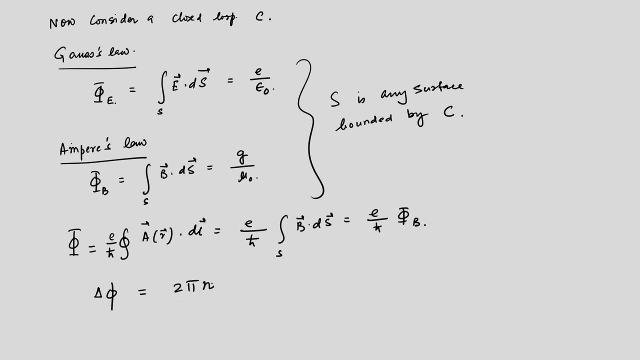 not pick up any phase. So the delta phi should be equal to some 2 pi into n, where n is an integer. ok, So this tells you that if the change in, so this is the phase shift of the wave function, and then this is delta phi equal to 2 pi n. now that tells you that the magnetic flux 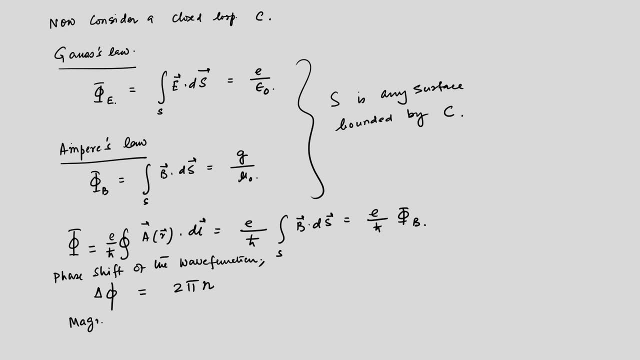 is quantized. ok, So phi b must be quantized. So that tells you your phi b is equal to 2 pi. h cross by e into n, which is nothing but h over e into n. ok, And so h over e is nothing but 2 pi. 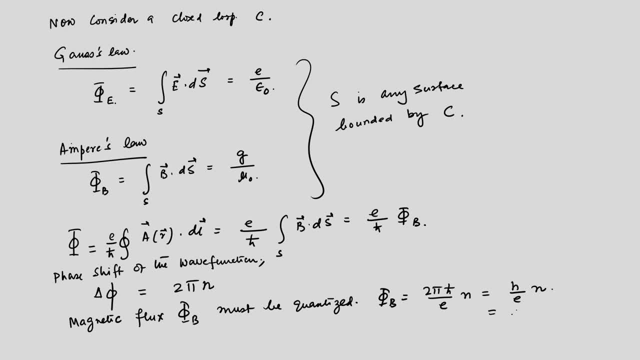 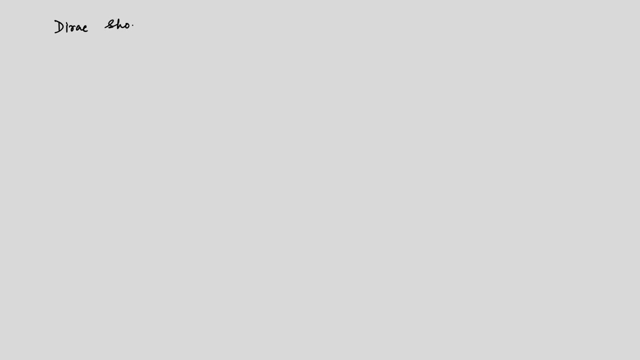 h. You know that is the flux quantum. So this is the flux quantum which is very familiar, and multiplied by n, So the magnetic flux will be some integer times the flux quantum. and in fact what Dirac showed, that this product of the electric charge and the magnetic charge, so this product of electric 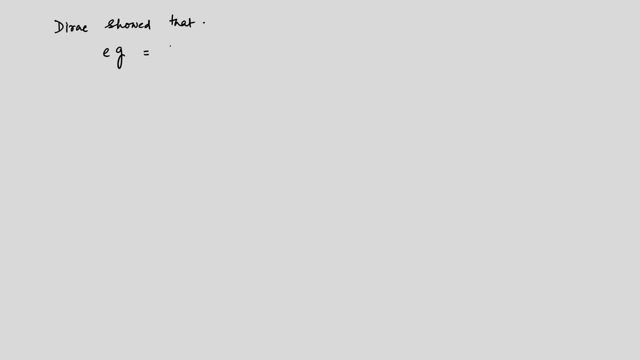 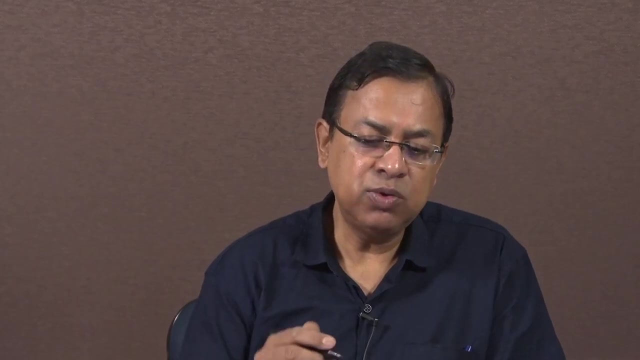 and magnetic charges and say this is equal to h over 4 pi into n, and this is the main result that he said, that these charges are quantized. So the existence of magnetic monopoles would explain the quantization of the electric charge and these integer n that you see is 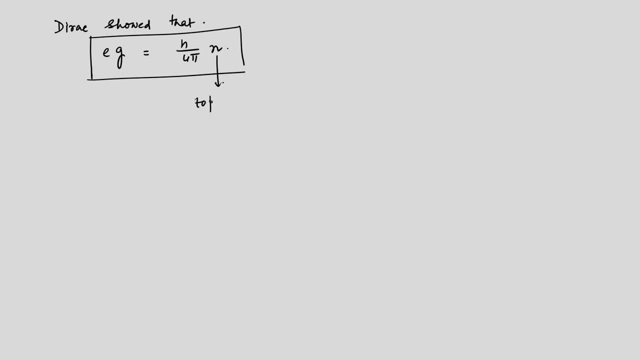 a topological quantum number, So it counts the number of windings around a singular point, and the singular point is the point at which the monopole resides. So the monopole actually acts like a vertex and you take the wave function or to take the particle around that and it 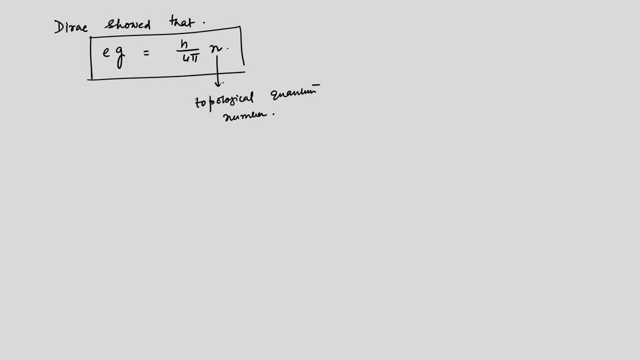 just counts the number of times it sort of winds, and these are also, you know, can in a sort of tight, binding model. we will see how to calculate that and so on, in order to calculate the topological quantum number, or which is called as a topological invariant. 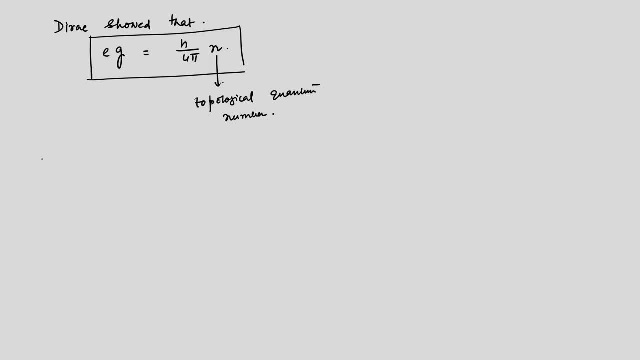 So the next is Aranov-Bohm effect. let us write S2.. So before this effect was, you know, first proposed as a thought experiment by Aranov and Bohm, and then, you know, it was actually verified in experiment by Chambers. 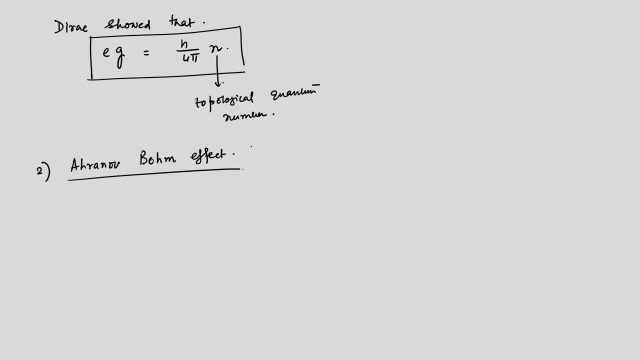 It was in 1960, so this was in 1959. yeah, so just about a year later it has been verified. So the burning question is that we know about fields- electric field and magnetic fields- and electric field corresponds to a potential such that E can be written, as you know, minus. 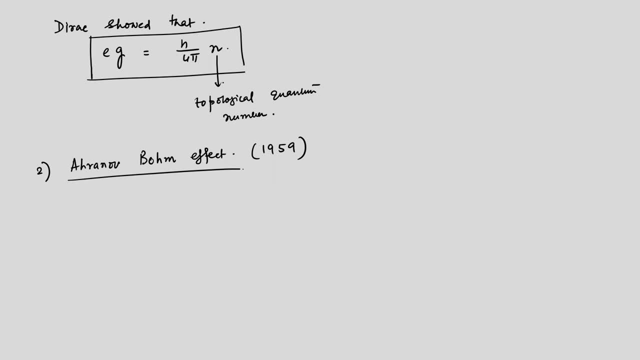 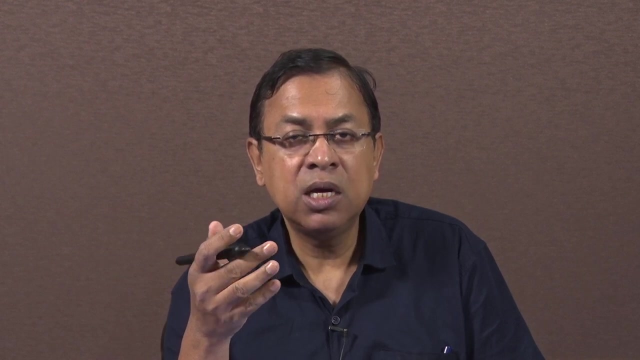 grad phi, and for a static case the curl of the electric field is equal to 0.. And And just other way around, the B has also sort of is represented by a vector potential, and this has no scalar analog, I mean in the sense that B is obtained from a vector potential. 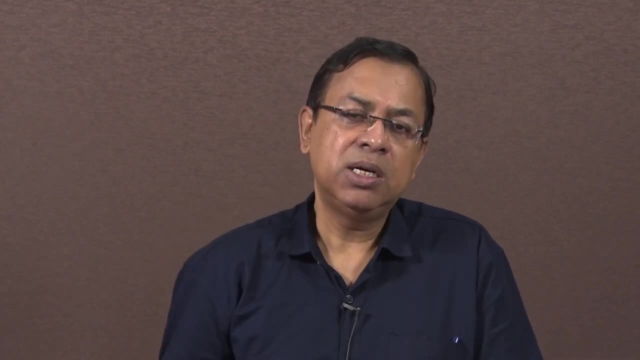 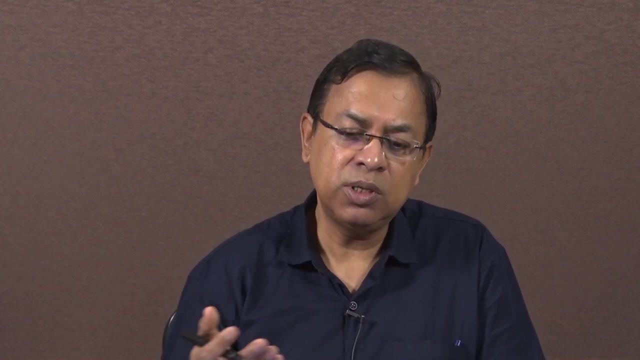 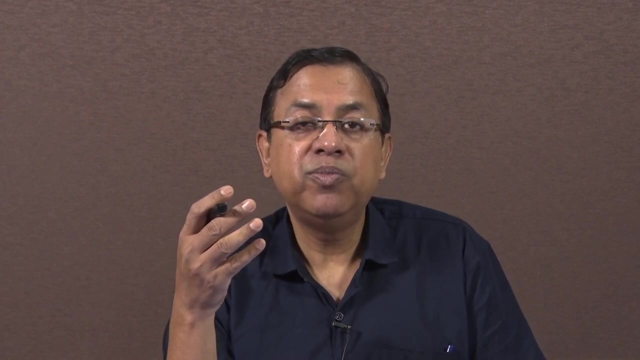 by taking the curl, So B is equal to curl A, and this is quite an important thing in the development of these Maxwell's relations. and I mean equations, say Maxwell's equations, and how the wave propagation etc were sort of you know from these, written down from these. 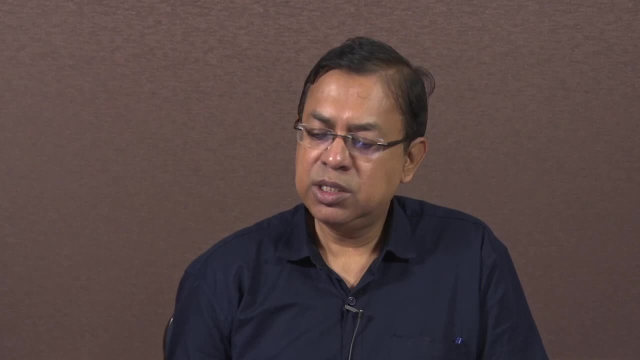 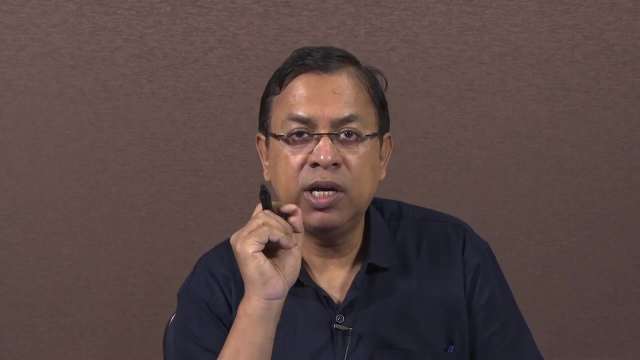 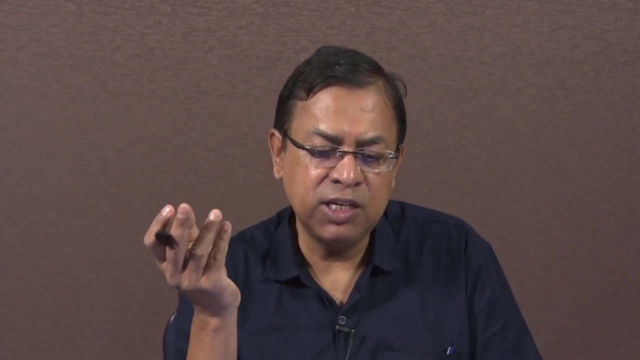 Maxwell's equations. However, it is Aronob and Bohm argued that is not the fields that are most important, it is the potentials, which are phi and A are quite important. In fact, they are more important than the fields and, in fact, the all the Maxwell's equations. 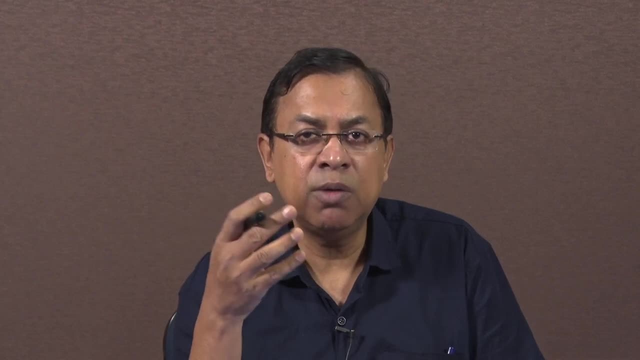 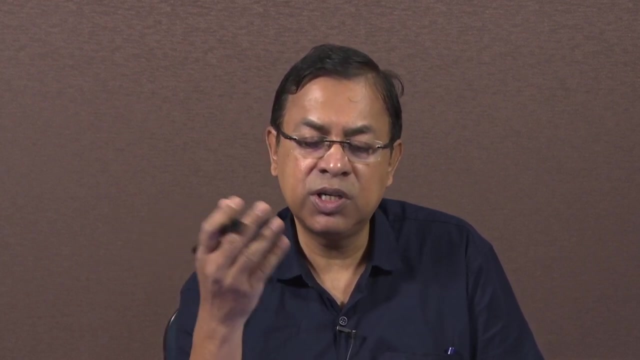 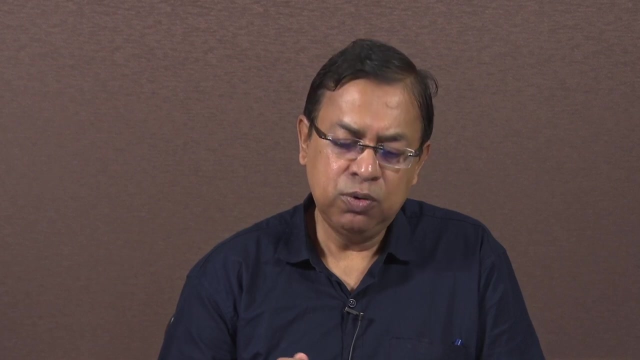 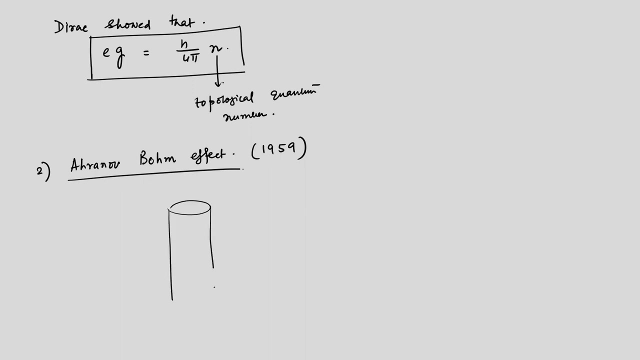 can be equivalently written down in terms of these potentials instead of the fields, which is more familiar to anyone you know working on this or studying physics. So, in order to you know, sort of pin down their views, they asked to consider: So this is like a solenoid, a very long solenoid, and so to show that it is long, that is like: 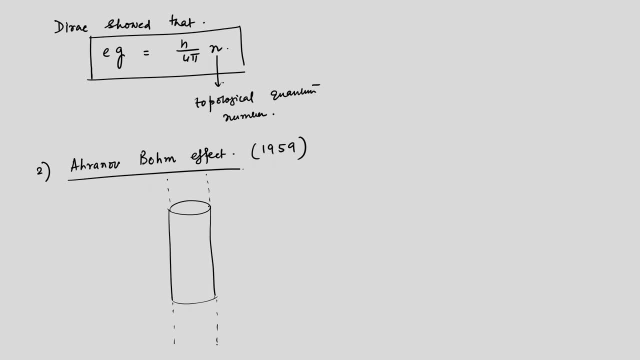 infinite this thing, we are showing this and there are these turned, the wires are wound around the solenoid, and why we have taken it to be very large is, or very long, is that we want to eliminate the edge effects Now inside the solenoid, suppose the current is I so 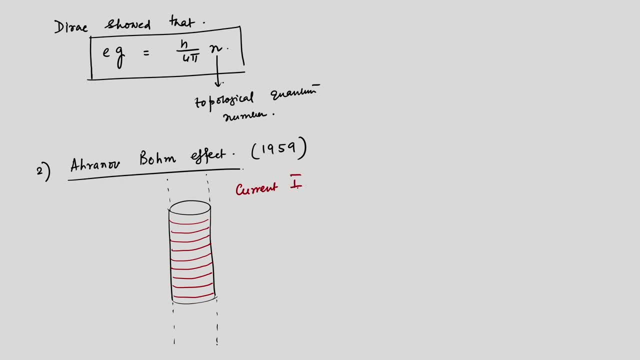 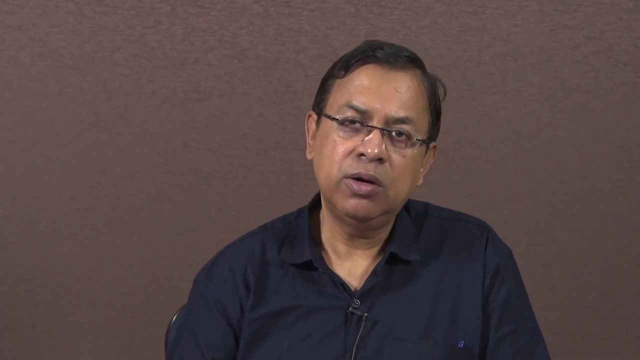 current I, which is going through the loops and wound around the solenoid, and this will produce a very constant or uniform magnetic field inside the solenoid and this magnetic field outside the solenoid is 0 and that is why we have taken, we have neglected the edge. 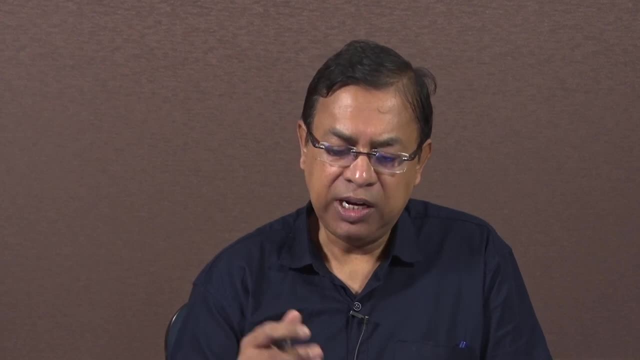 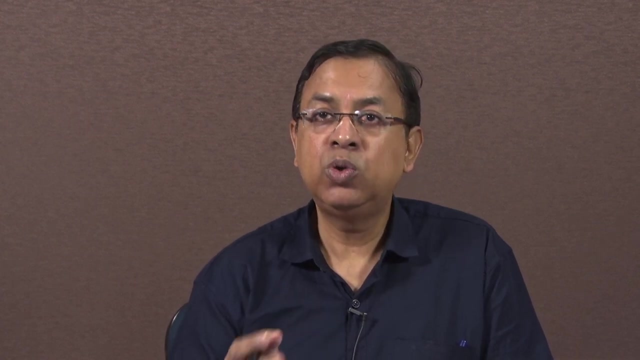 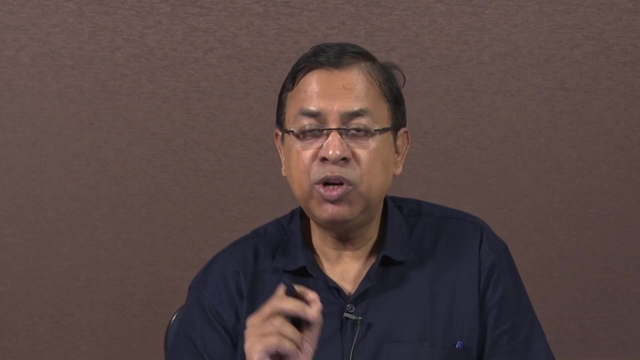 effects. So we are talking about that. we are, you know, talking about a very large solenoid. So inside the magnetic field is non-zero and uniform, outside it is equal to 0, but outside it is equal to 0 does not mean the vector potential is equal to 0. In fact, the vector potential 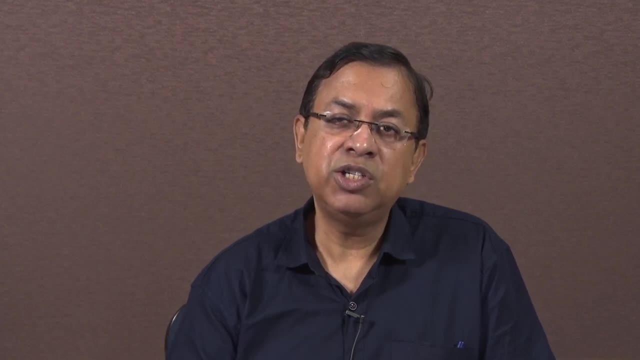 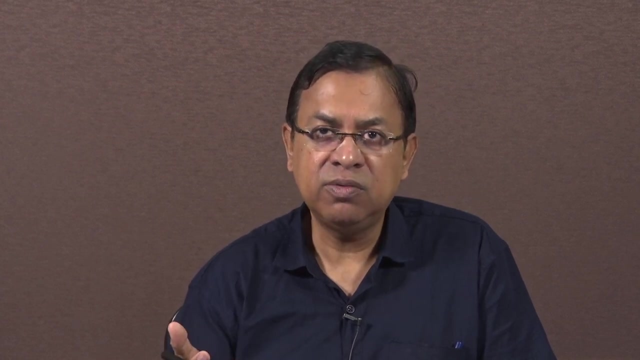 exists such that the curl of the vector potential vanishes. and we know that when curl of a vector vanishes, that means it is an irrotational vector, Which means that it does not rotate, it does not curl, it is like a vector that is you. 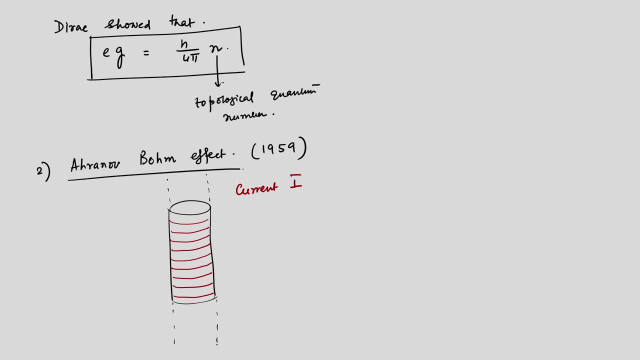 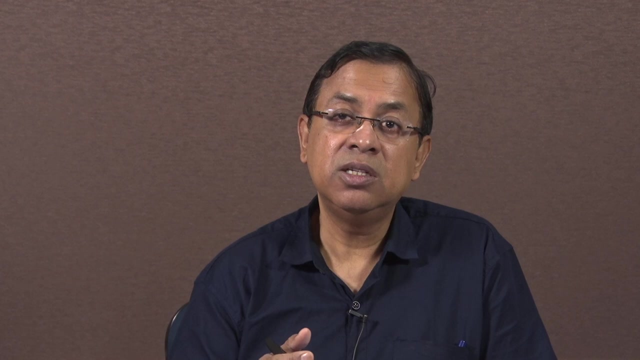 know, either increasing monotonically, or decreasing, and so on, so forth. So nevertheless, I mean, the whole assumption is, or rather these finding, is that even though the magnetic field is 0, the vector potential still exists. and how would we know that the vector potential exists? 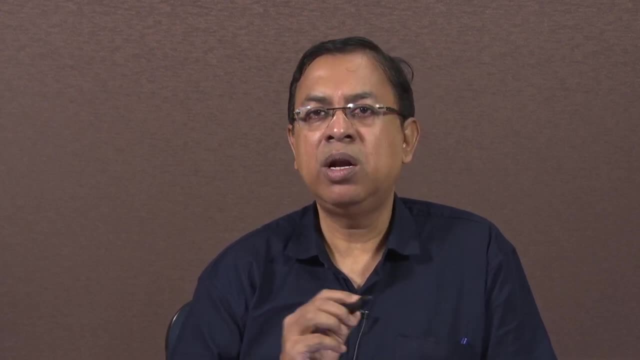 So suddenly the position is so large, the position is so small that the potential is zero. So how we know that the, the vector potential, exists? So we have taken these two. one can send one electron from one side of the solenoid. suppose you are having this solenoid. 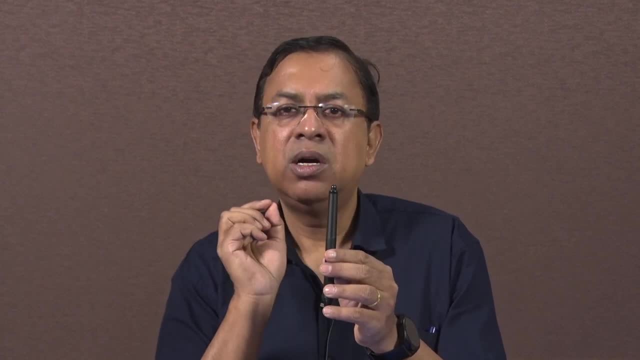 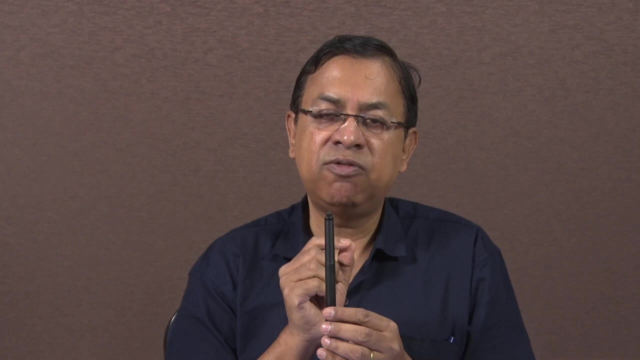 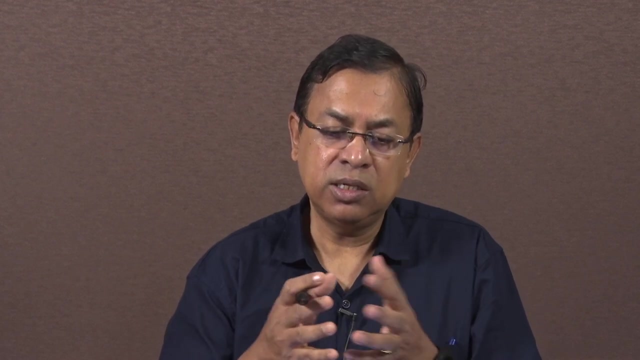 one can. one electron can be sent from the right of the solenoid and go and hit a screen at some distance away, and another electron can be sent from the left of the solenoid and would again go and incident on the screen at a distance, at a certain distance away. now, these two electrons. 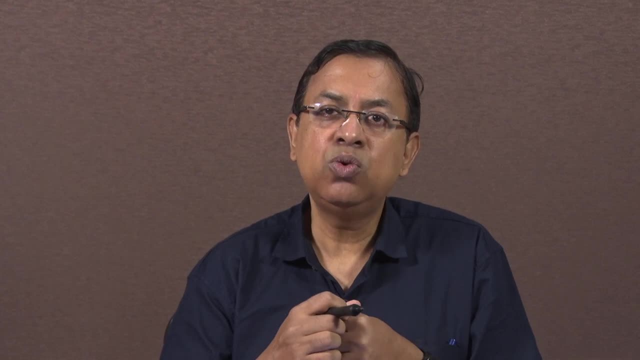 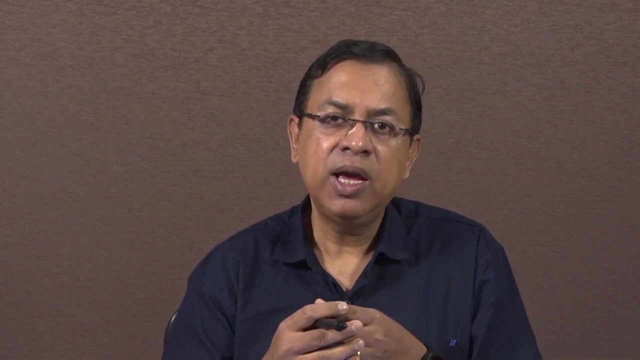 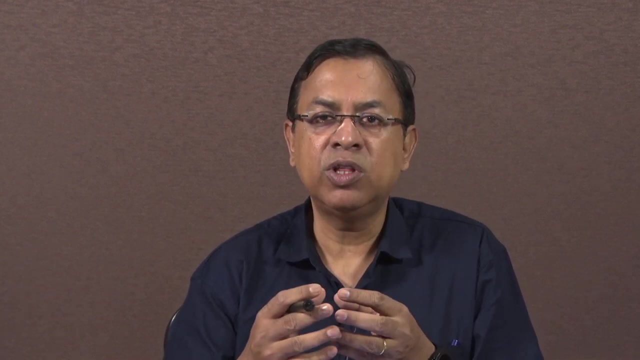 they also can be considered as waves and these two waves, when the incident would have a different phase, okay and the, it will have a constructive interference or a destructive interference, depending on the phase relationship between the between the two electrons, which goes to theasia, solenoid, but they have to be considered the same. From top to bottom. you could have drawn a kind ofnapike, an incident with two electrons without tresential derivative with it. It is like to have dediromatiza, introducing all the above elements at the same time and, in theنone, pancakes added, which has also been conducted in the 나오omar report. 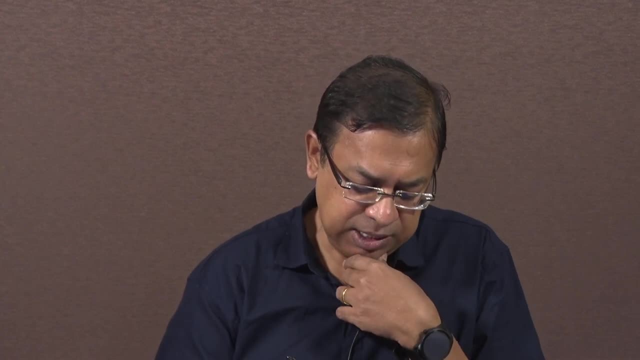 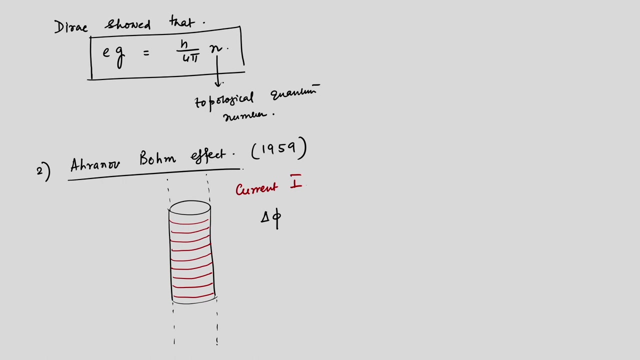 goes from the left and the right and this phase difference can be obtained, or rather it is finite, because the vector potential exists and this is equal to E over h, cross and AR, dot, dl, where dl is the length that it travels and A is the vector potential that 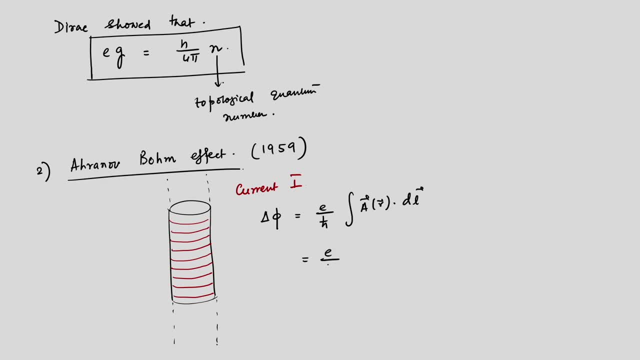 exists, and this is again by using nothing but the Stokes law. we get it as B dot ds. So this is, you know that, curve C and this is that S it is a B dot ds. okay, So this is the thing, and one can actually verify it in experiments, which Chambers did in 1960. 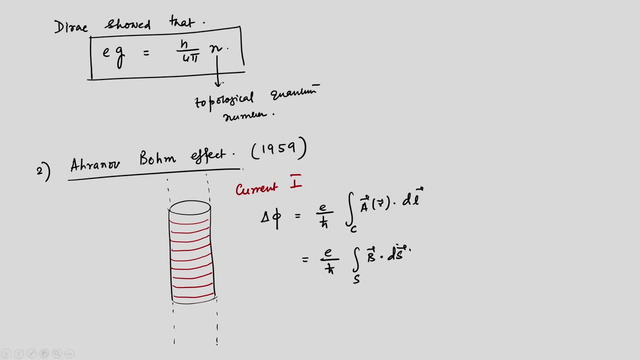 Now this is a very important thing- that if this is a measurable quantity and this actually verifies, It verifies in experiments, which means that the potentials are more important quantities than just the fields, and in fact this was earlier not known. So what is important here is that you know the solenoid actually contains, or the singularity. 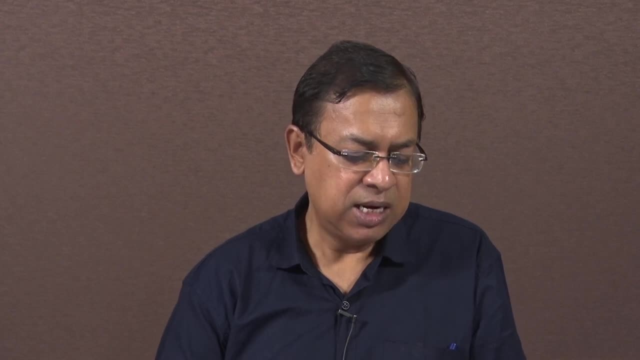 in the vector potential. It is like a vortex, as we have said, and then you can actually view the solenoid as a hole in the space which is allowed for these vectors. Okay, So the quantization arises from the fact that the curves in the space of A, the 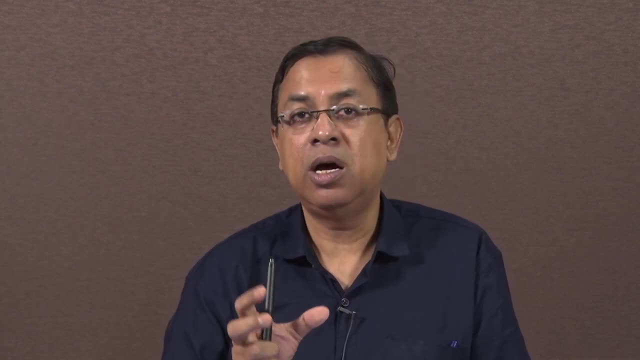 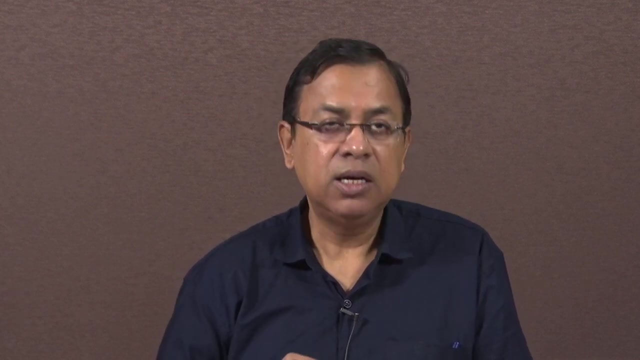 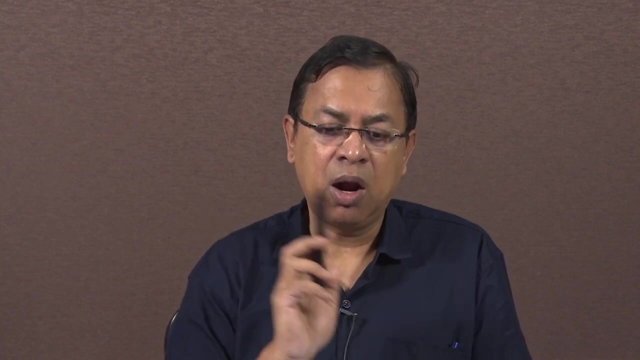 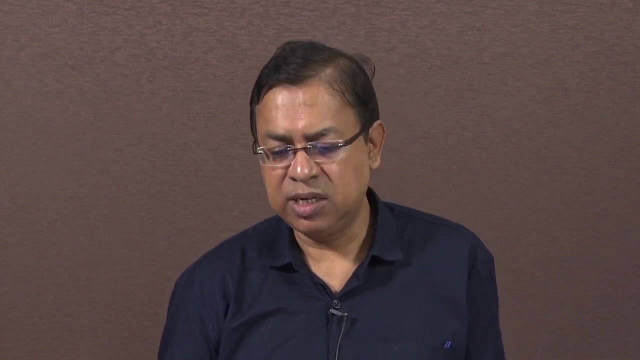 vector potential that encloses solenoid are noncontractable, okay, So they cannot be contracted, and so on. and the winding number thus produced, which is a topological invariant which is taking these particles around the solenoid, Okay, these winding number characterizes, you know, the distinct homotopy classes, etc. 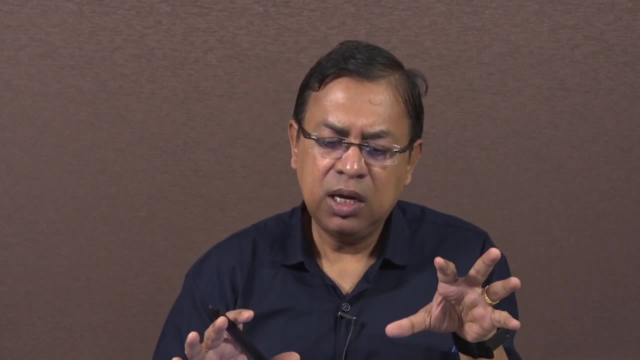 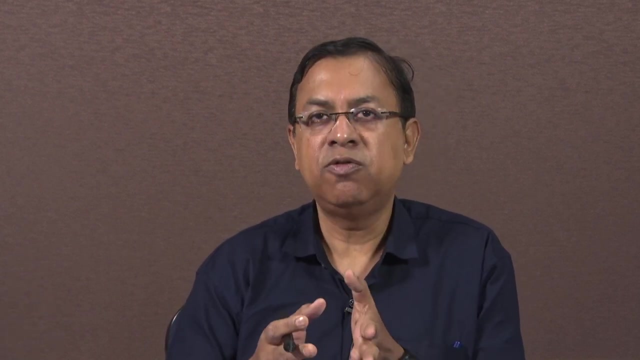 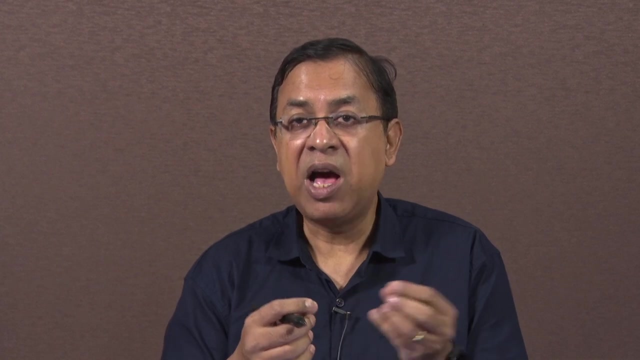 So what I wanted to make sure is that as soon as there are these systems with singularities or vortices- here, for example, this- there is a vortex which is coming from the solenoid itself and the magnetic monopole is just like a vortex or a singularity at its position. 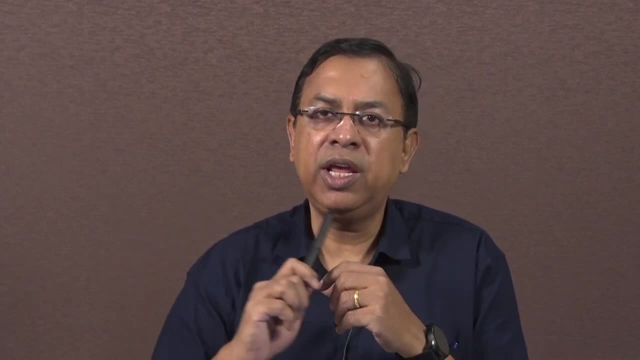 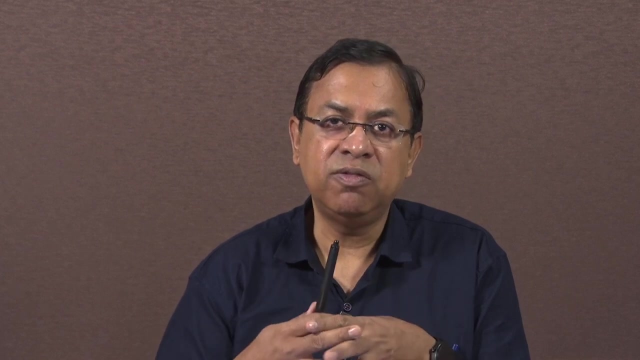 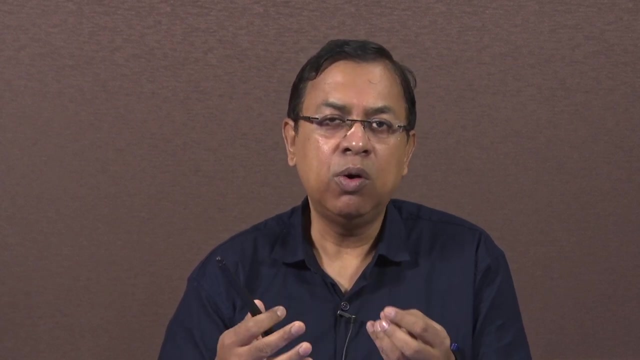 So there, when you take a charge or take a particle, you know around it it will give rise to quantized effects, and this is the topological quantization that one is talking about. So this will not go away, even if you know you can adjust other quantities and this will. 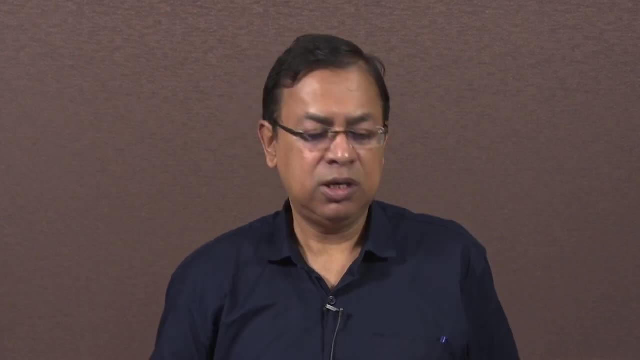 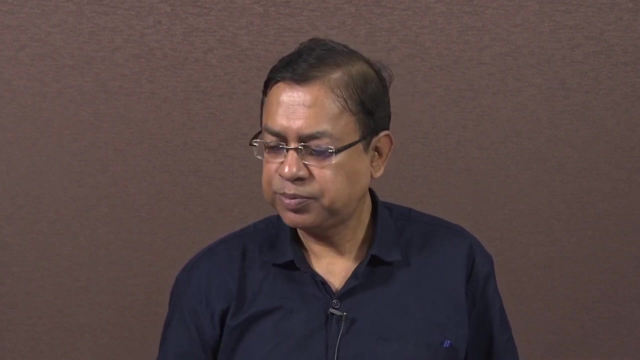 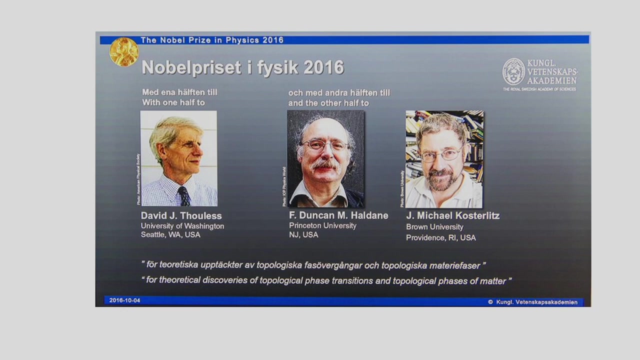 still remain. So Aronoff-Bohm phase is an important. it is a sort of indication of topology playing a role In this simple thought experiment. ok, So let us come to physics and let me, you know, show you- I have already told you this- that. 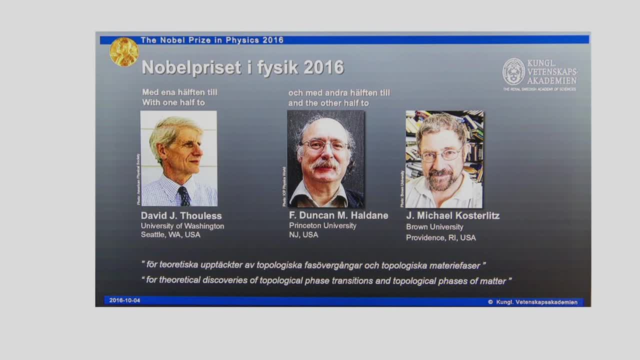 this 2016 Nobel Prize was awarded to for the theoretical discoveries of topological phase transitions and topological phases of matter. these are by David Thouless, who won half the Nobel Prize, and the other half went to Duncan Holden and Michael Kosselys. 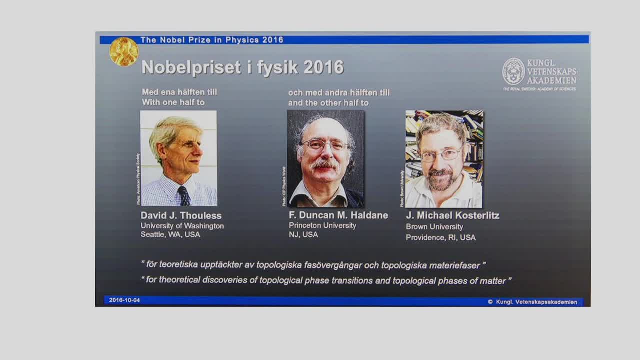 I believe, David Thouless and Michael Kosselys. they were awarded for the topological phase transitions, whereas the topological phases of matter was due to Holden- Duncan Holden- which he showed in the mid to late 80s through a number of you know very well cited publications. 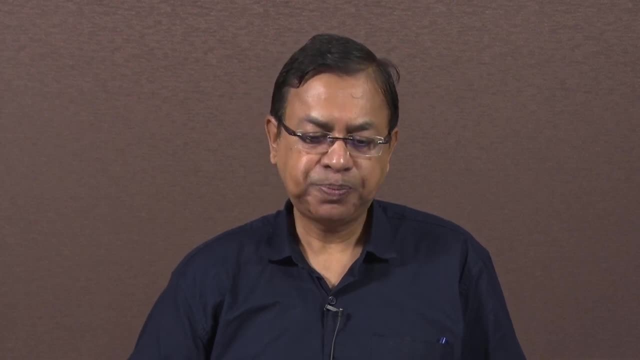 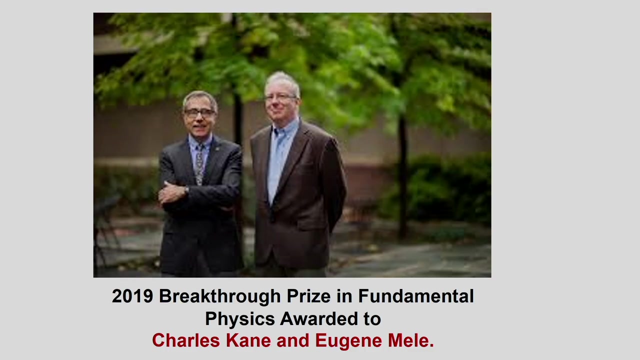 We will talk about what is called as a Holden model, etc. And this was in 2016 and after that it was these two gentlemen who had popularized again the concept of topology. It is not popularization, it is more like applicability and into this quantum spin Hall phase. and they 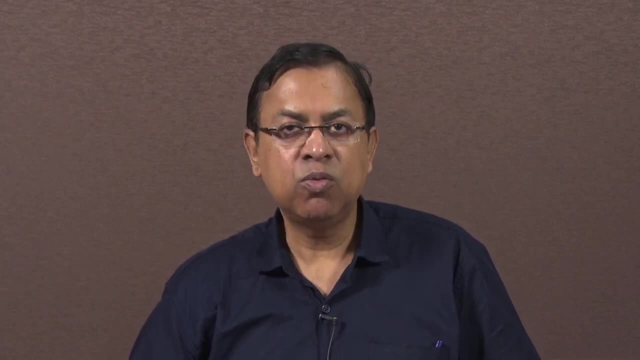 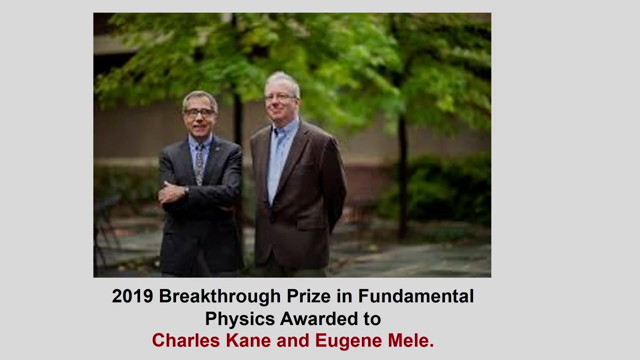 have written down Hamiltonian, which does not have quantum Hall effect, but it has another topological invariant called as a Z2 invariant, and this is non-zero. They won at 2019 breakthrough prize in fundamental physics, awarded to Charles Kane and Eugene Milley. 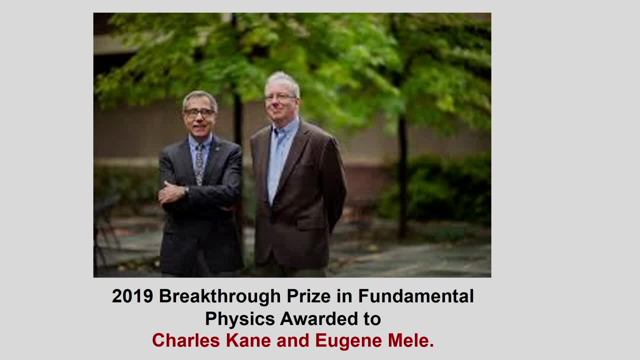 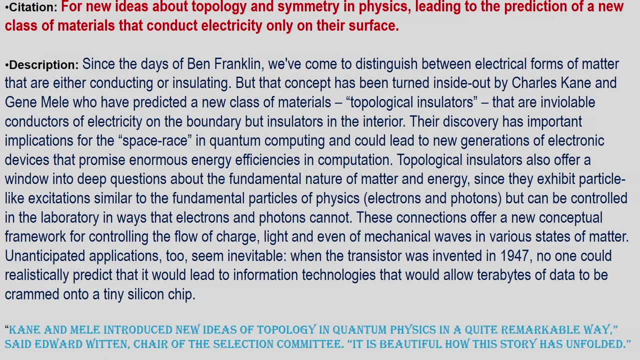 Charles Kane is on your right and Eugene Milley on the left. Let me read out the citation. it is very interesting. particularly it is you know. it predicts that there would be a lot of applications of these proposals From Kane and Milley on the quantum computation, quantum information, etc. and quantum technologies. 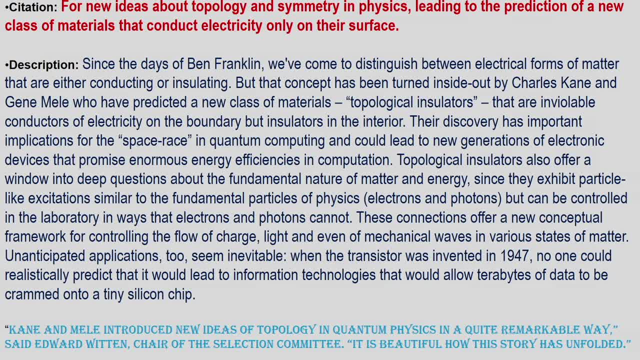 So the citation says that for new ideas about topology and symmetry in physics, leading to the prediction of a new class of materials, which are the quantum spin Hall, materials that conduct electricity only on the surface, and this electricity is actually the spin polarized current. Okay, 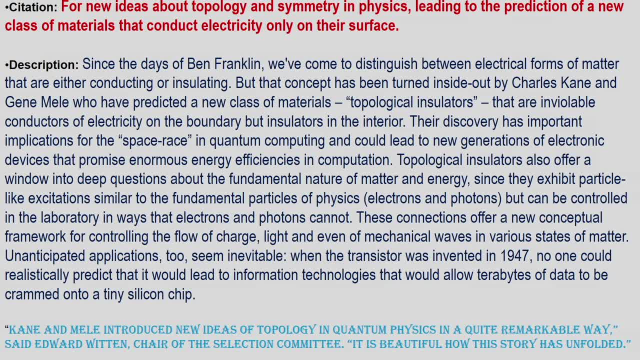 The description is quite interesting. let me read it out for you. Since the days of Ben Franklin, we have come to distinguish between electrical forms of matter that are either conducting or insulating. But that concept has been turned inside out by Charles Kane and Eugene Milley, who have 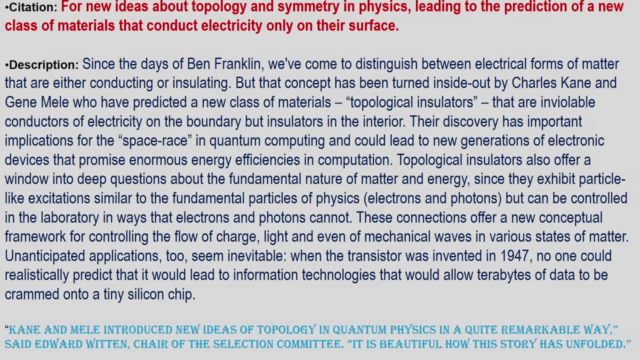 predicted a new class of materials, the topological insulators that are inviolable conductors of electricity on the boundary But insulating or insulators in the interior. so these very fact that they behave differently at the edges compared to the bulk. if you look at this board, that you are the screen, that 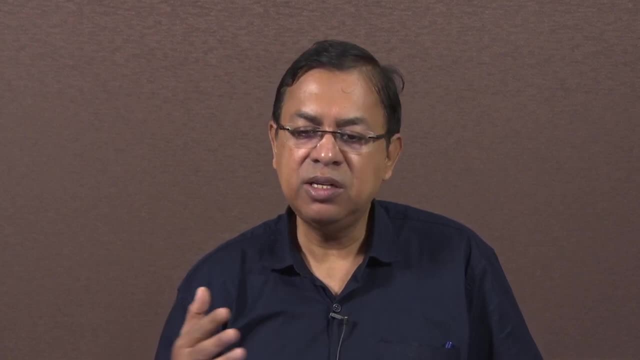 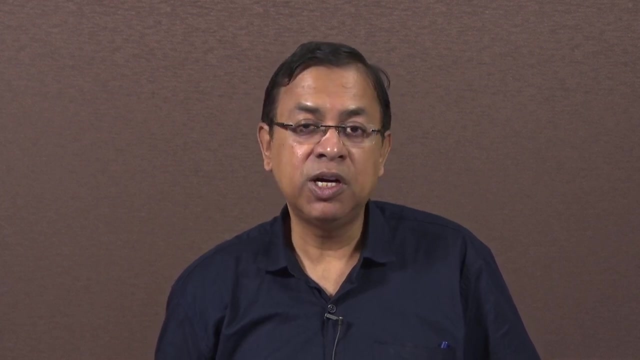 you see, if I have these screen, the edges of the screen, that behave differently than the bulk, I would not feel comfortable about it. In fact, most of the systems that we know, they have no distinction between the behavior of the bulk and the edges, and this is what precisely makes these things so interesting. 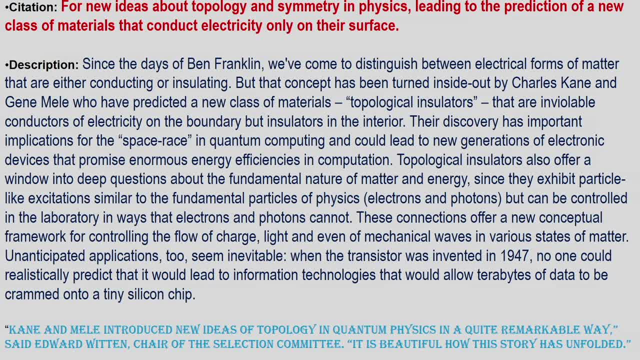 So the discovery has important implications for the space race in quantum computing and could lead to new generations of electronic devices that promise enormous energy efficiencies in computation. topological insulators also offer a window into deep questions about the fundamental nature of matter and energy, since they exhibit particle like excitation, similar 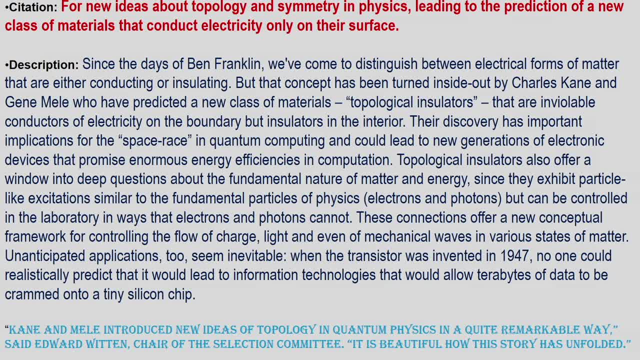 to the fundamental particles of physics- electrons and photons such as them- but can be controlled in the laboratories in a way that electron and photons cannot be done. These connections offer a new conceptual framework for controlling the flow of charge, light and even mechanical waves in various states of matter. 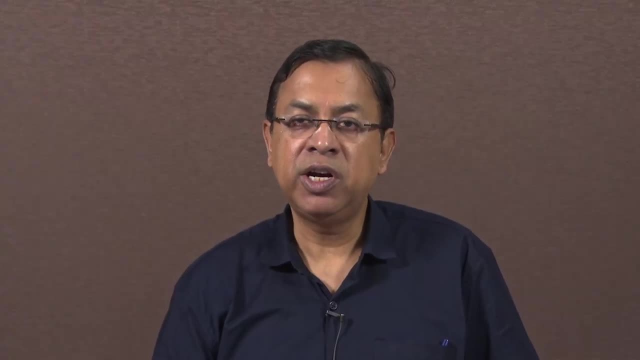 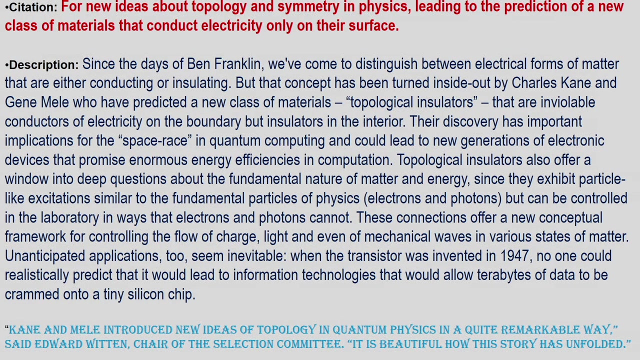 This is what I was saying. I was saying that topology has proliferated beyond electromagnetic theory or optics or condensed matter physics. it has entered into acoustics. it has entered into mechanical matters, mechanical sort of materials and various other things. I mean unanticipated applications to seem inevitable when the transistor was invented.